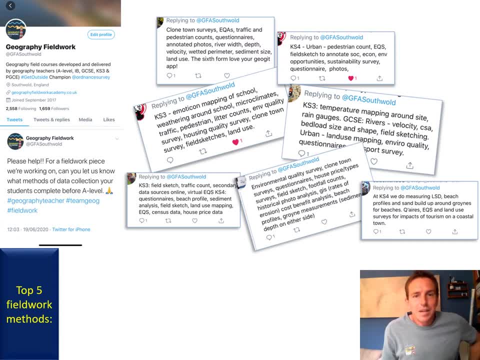 students across this country and it's useful for us, as I say, to gain a bit of an understanding about what things you guys are doing, and what things you've done, and perhaps also what things you haven't yet done and therefore, what things might be useful for us to introduce you to So number. 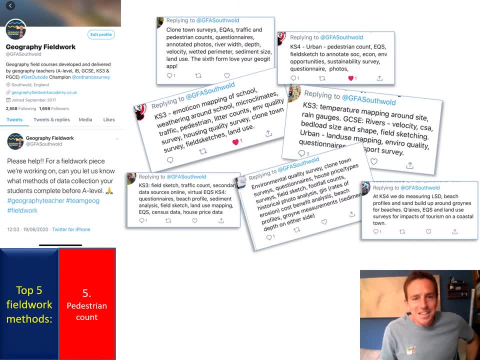 five on the most popular charts is the classic pedestrian count. an absolute beauty. this, this is where you count people. You might do it over five minutes or over one minute. you might be unlucky if you're told to do it over an hour. that could be a bit boring, but a pedestrian count is a. 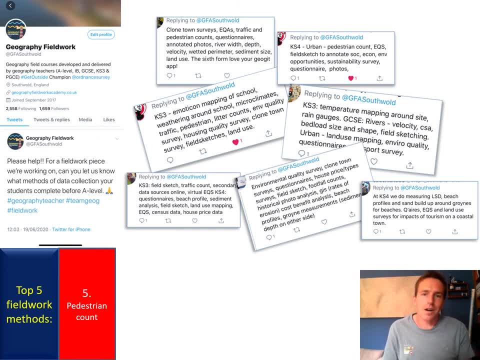 data collection where you kind of gauge how popular an area is or how unpopular it is. This might be useful if you're trying to assess the success of something like a regeneration project or town centre, and it's a pretty basic thing to do and it's a fairly straightforward thing to do. 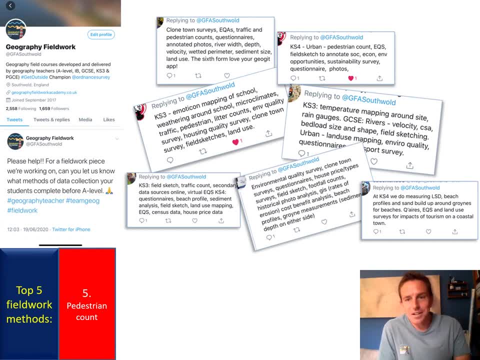 I know my daughter, who's six, did a pedestrian count in our local village and just before lockdown and she said that it was. it was quite an interesting, exciting thing to do as she counted all of the older people making their way to the butchers and the bakers. 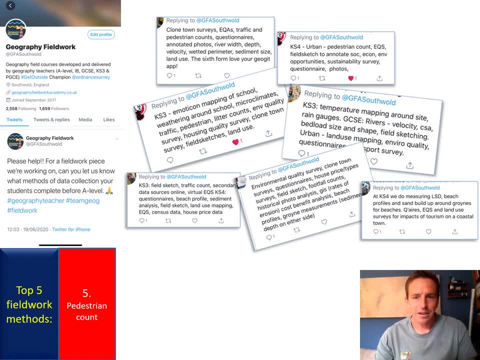 So there we go. it's a good one to use and there's still value to including a pedestrian count at A-level, just depending how you use it. The fourth one on the top five charts is a land use survey, and a land use survey is also a very traditional form of geography data collection and very often 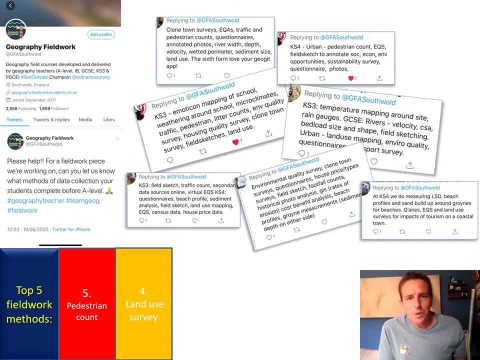 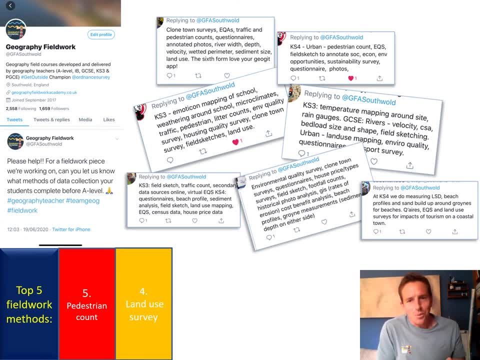 residential, industrial, commercial. I'll stop there before I get get it wrong. I think it might be entertainment next, but the idea is that you have these different distinctions of land use and when you're in different areas of a particular space, you you make a judgment as to how that area best. 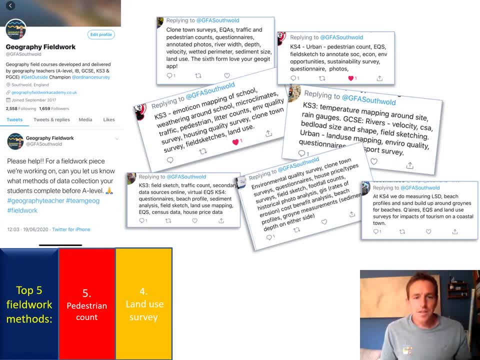 fits into one of those eight different land uses. So land use can change over time and obviously it can change depending how far or close you are into the middle of a settlement or development. and it can be quite an ideal, Ideal form of qualitative data to get an idea about different functions of a place. Third one is one that 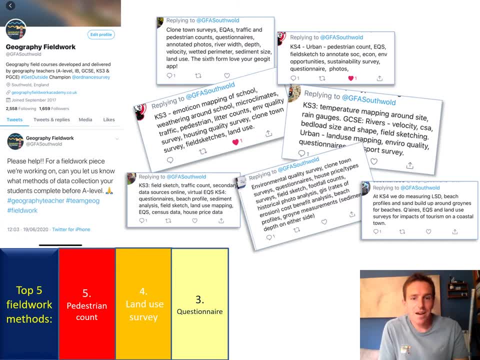 some people dread, some people embrace and love and end up having conversations with people who turn out to be, you know, lifelong friends. Questionnaires are ones that have been around for a long time. doing a geography questionnaire is often something that your your parents will probably talk to you about when they think about fieldwork, and and and. 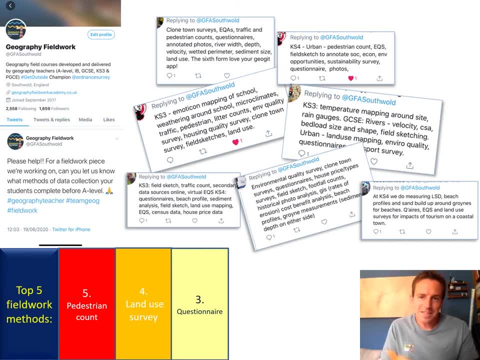 I would say that, although there might be some cases where you might fear doing a questionnaire, that actually speaking to people is very often the best form of data collection and if you do have the confidence to speak to people and organize questions that are appropriate and crucially relevant as well to what it is that you're hoping to find out- Questionnaires and 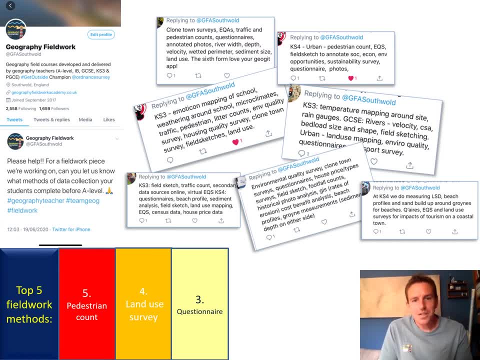 the interviews are a magnificent source of information and there are ways in which you can use this information: by kind of coding the results that you get and the articles that you get, that you get, or presenting them in a variety of graphs. questionnaires definitely still have a place in geography fieldwork Now one of the 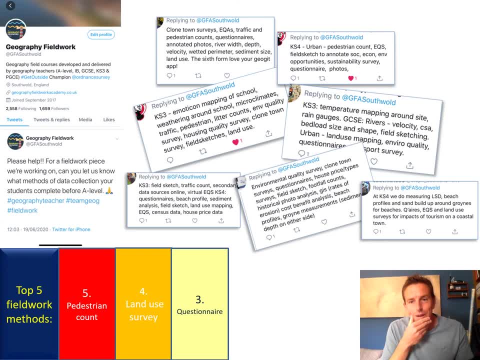 things that we might be able to do over recent- not over the coming months- is be a bit more creative about how we get this information verbally from people, and it might well be that you could do zoom interviews with people that are going to be relevant to your study, or it could be that you develop things like 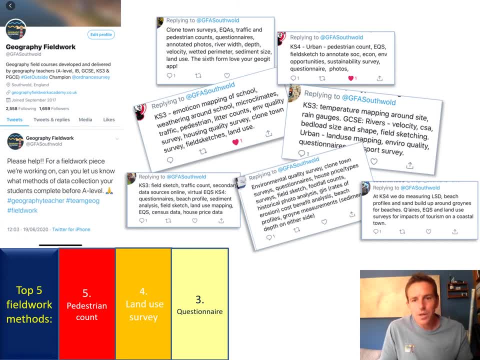 online surveys. maybe you can make a questionnaire on Google Forms or on Survey Monkey and then you can attach this questionnaire on to an online forum like Facebook or nextdoorcouk, and that may well be an appropriate way of you gathering your questionnaire data, so don't rule that out. it could be. 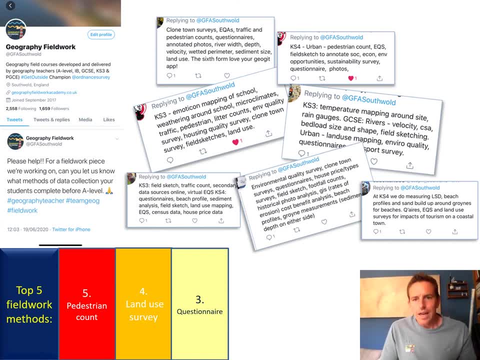 that we're just a bit more creative about how you gather your questionnaires. So we come down to the top two. this is getting tense now. which are going to be the top two most popular questionnaires, Top two most popular methods of fieldwork data collection? Well, the second one. 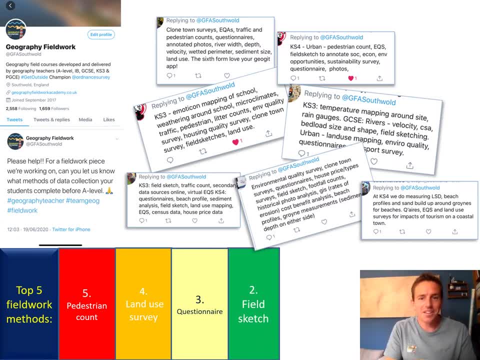 surprised me, but I'm glad it's there. the second one are field sketches. Again, some people might think I'm rubbish at art. I picked geography, not art. I can't draw, doesn't really matter. In geography you're not marked on the quality of your 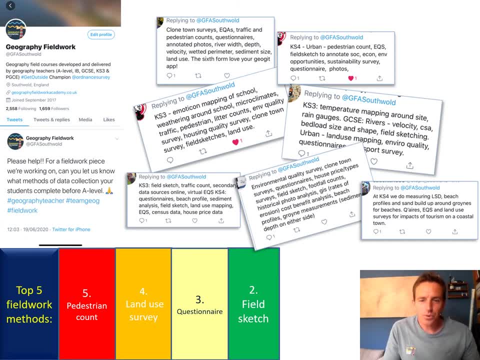 actual drawings. it's more about the quality of the annotations that you add to your drawings, and your field sketch is literally where you're just trying to get the basics of the landscape that's in front of you down, and there is a still definitely real value to including field sketches, but in 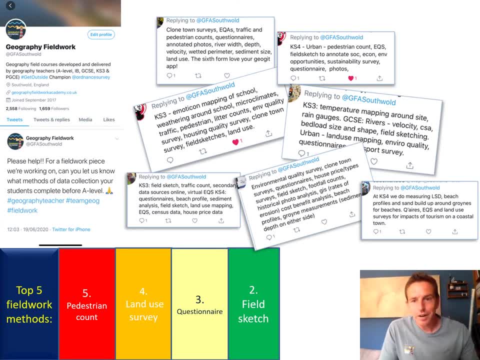 addition to that, most of you have got a smartphone in your pocket that has got a very good camera on it and taking pictures of the landscapes that you're investigating and then later using those pictures and annotating those is just as good as a field sketch. and so you know, don't be afraid to use annotated photos. 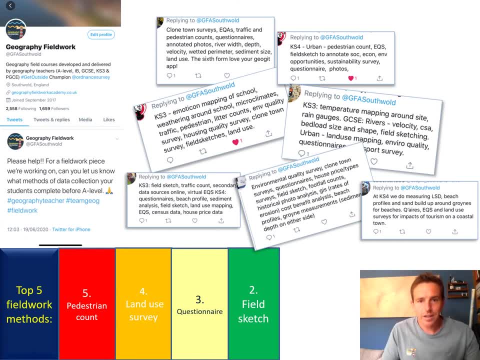 or field sketches in an A-level study. they're completely appropriate and actually even at university level, students are taught the skills of doing field sketches, So I think that's a really good way of doing field sketches. So number one here, it is the top method of data collection for. 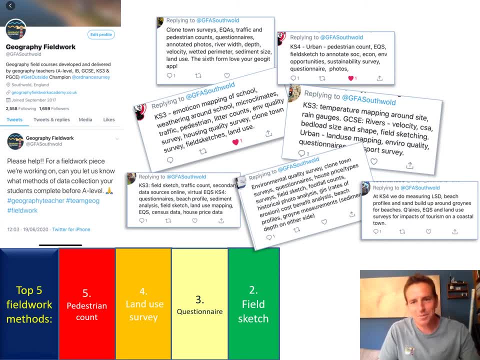 fieldwork for geography students in the UK is currently, according to our short survey, the classic environmental quality survey, or EQS as the fans of this method like to call it. An environmental quality survey is a way of gauging- as it's kind of the answers on the tin- really- the quality of the environment in the 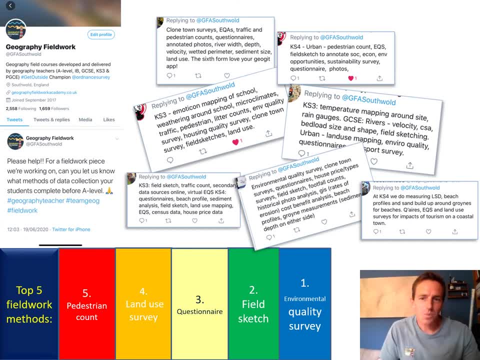 number of different locations, and there's a huge amount of ways in which you can design this and lay it out. I'll show you a couple of examples during this session, but this is a very much a method that you can make bespoke to you by adding your own criteria, your own scales, and you'd also, when you were doing an 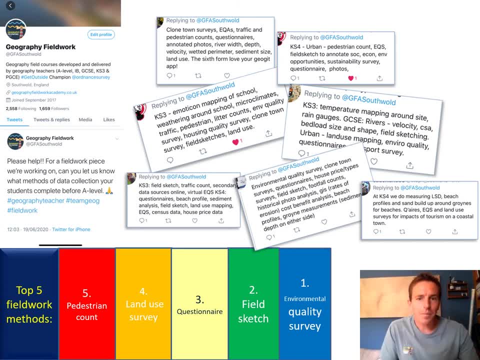 environmental quality survey. key thing to remember about an environmental quality survey is that it's all relative, and if you only ever do one of these, then that's not enough. you need to perhaps have a perspective where you do one in one location and you compare that to another location. so an 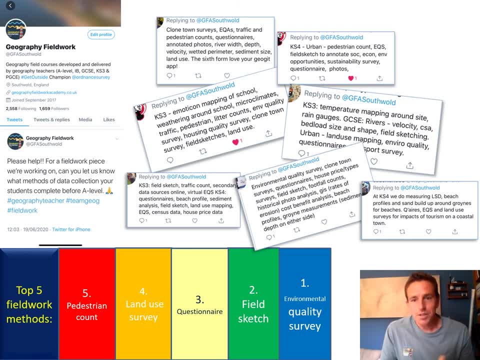 environmental quality survey gives you in total. what an overall score about the quality of the environment in one place. but that's only really useful if you can then compare that to the quality of the environment somewhere else, and the best environmental quality surveys are where you do that in lots of locations. so you 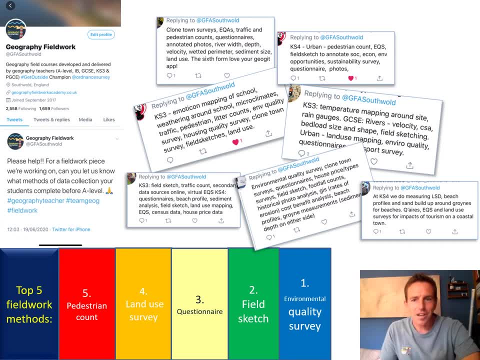 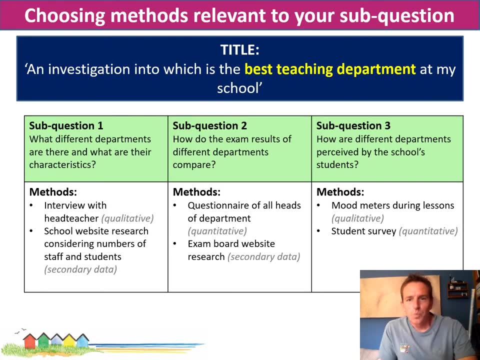 can see how that changes across across a given location. Okay, so that gives us a bit of an idea. Going back to this page, then, this was one of the slides that we covered in the previous session, in session three, and I said that this is the very kind of basic. 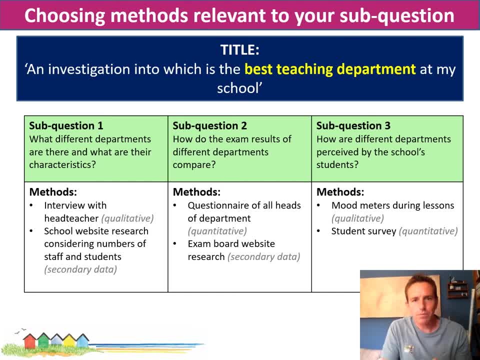 structure or template of designing a geography report, and we said, obviously, that your first challenge is to come up with your title, having picked the issue that you want to investigate. then you have these supporting sub questions and I said that most students will pick three. it might be two or four, but most 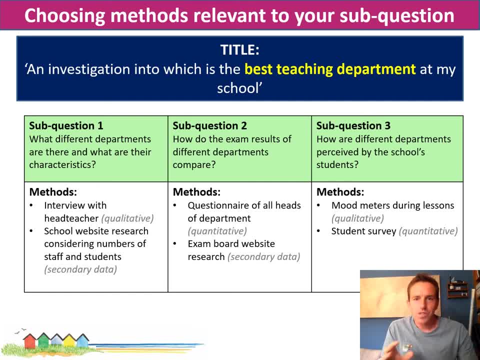 most students pick three And then your challenge then, once you've got these three sub supporting questions, is to come up with appropriate methods to answer those sub questions and to allocate methods to those boxes there that you've got When we showed you this example. here we're talking about kind of a mock example of somebody doing a, an 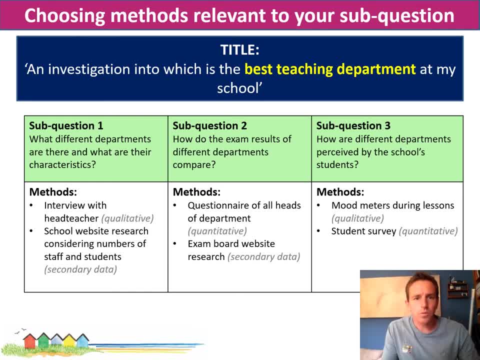 essay on the best teaching departments at their school, and you can see in the boxes there it says methods- that they've allocated two different methods to each sub question, and again, I suggest that might be something that you do. it might well be, though, for one of your sub questions you just have one. 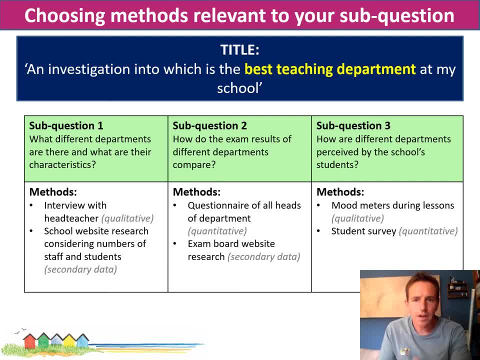 method. it might be that your questionnaire or an interview covers it and you don't necessarily need to have two or three methods to answer that one sub question. but holistically, when you look at the methods that have been chosen overall, there should be a mixture between qualitative and quantitative. so 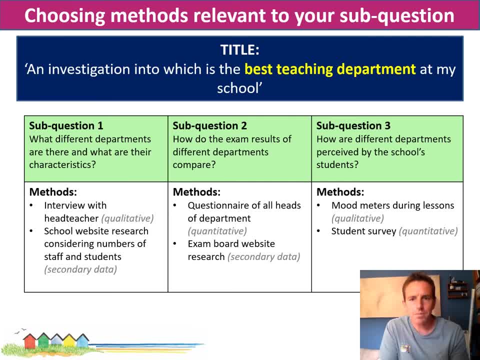 numerical based, counting or monitoring Most measuring surveys and there should be some that are gathering more qualitative or written or wordy responses. so we've got those kind of qualitative quantitative mixtures. it doesn't have to be a complete balance, and the other thing that you'll probably expect to find more of in the NEA's that 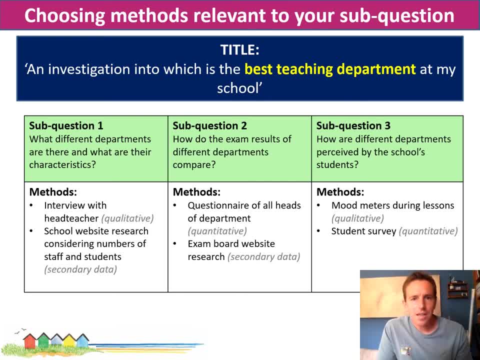 are going to be issued for your year. this, this coming year, is that it will probably be more secondary data supporting your primary data than on previous NEA submissions, and so you will need to then think again, with these sub questions that you've got, what secondary data can you gather to? 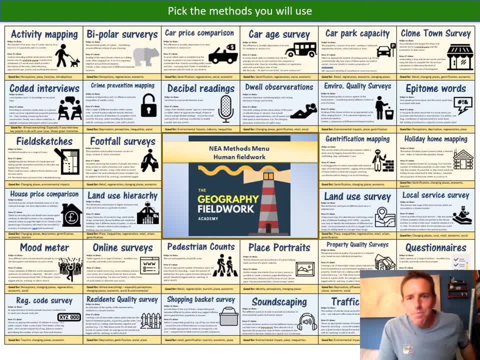 help you answer that question. So, with that in mind, your challenge at this stage, then, is to pick the methods that you will use, and the exercise that we did at the start of this session kind of showed that most of you guys have probably done five or six methods of geography fieldwork in your GCSE, and 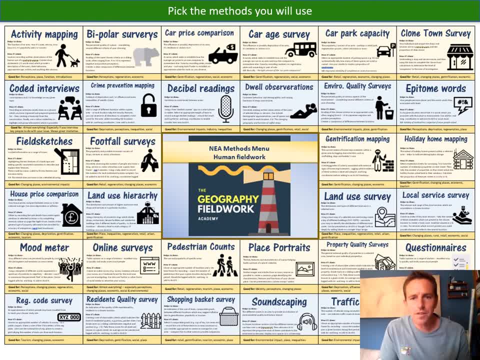 Key Stage 3 career so far. so you have been exposed to some methods, but you're going to want to have more of a menu, really, of methods that you can pick from and consider when you're planning your NEA, and so this, this is one of the things that we've put together. you'll find this on our website. we've 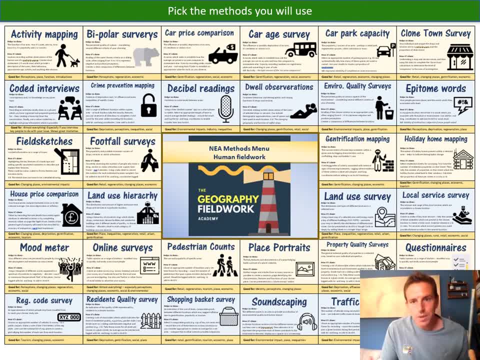 got this document where we've highlighted some other human methods of data collection and you can kind of look and zoom into those methods and, although it might be quite difficult for you to see on the screen at the moment, when you have a look at the kind of the PDF version of this document, you'll be able 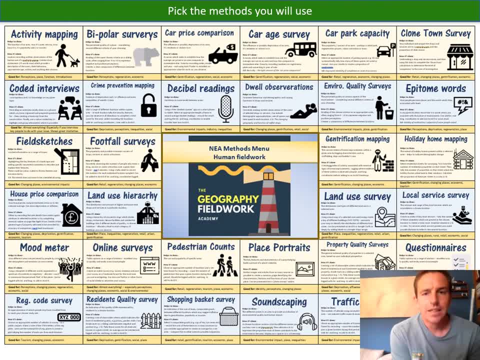 to see that underneath the document you'll be able to see that underneath the name of each of those methods there, it describes what that method is, tells you how you could use it and also in which scenarios and which studies those methods might be appropriate. so in total there I think there's about 25 different. 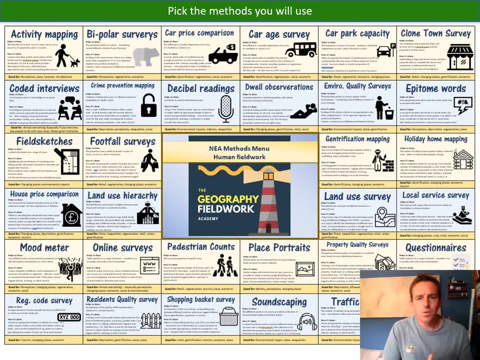 human methods. it's not an exhaustive list at all. there are definitely more methods of data collection that you can use in addition to the ones that are shown on that methods menu there. but that will perhaps give you an idea about some of the other methods that you can use in your GCSE and Key Stage 3 career. 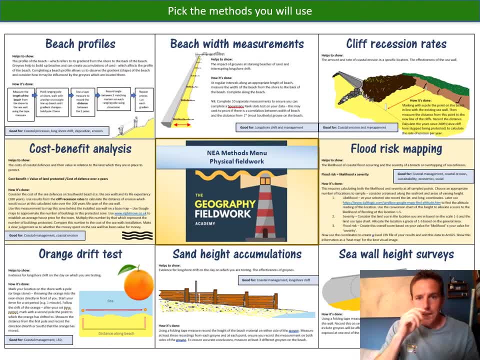 haven't used before and things that you could perhaps consider. another thing that we've also got on our website are some coastal methods. so these are some of the ones at a selection that I've just picked out and just kind of made those a bit bigger and again. with those there's a bit of a description about how. 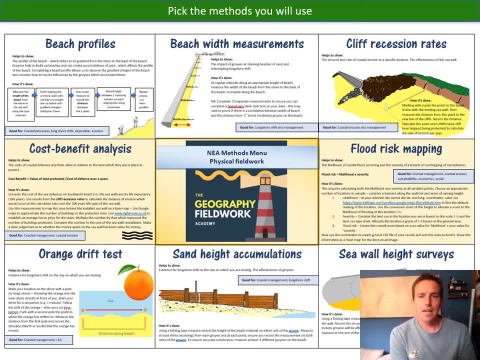 you could gather those methods of data and then, when it might be useful to use those, depending on what kind of studies you're doing. so there are a fair few ideas available on this website for you to use if you're interested in learning more about these methods. 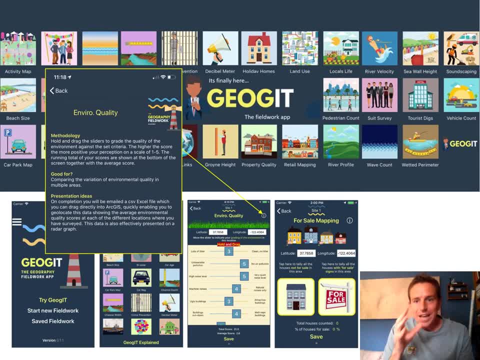 have a look at and to consider. I'll say, though, another thing that we will do a session on as one of these kind of virtual lessons, is on using technology to gather your geography fieldwork, and one of the things that we have spent a lot of time on a couple of years ago was trying to develop the first proper geography fieldwork app. 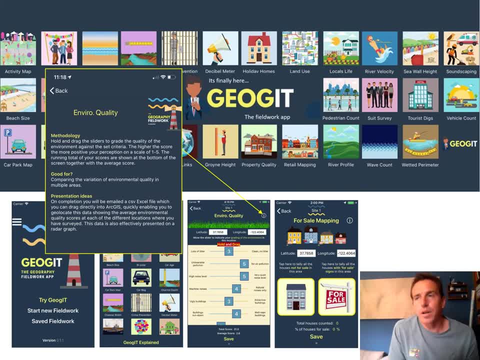 and we have now- it's been up and running for over a year. this is jog it, and jog it is the kind of designated fieldwork app, and on jog it we have loaded up 35 different methods of geographical data collection and essentially what this means is that 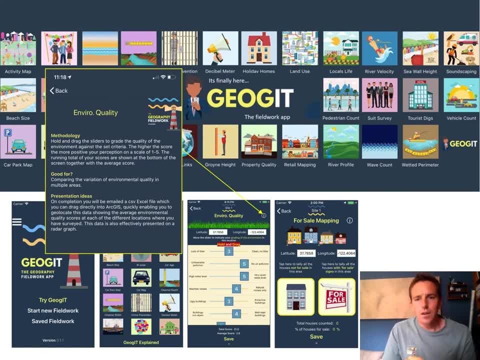 on your phone, whether it's an Android or an iPhone. you can actually be collecting your data directly onto your phone. you can be storing it on your phone. it then gets built into a behind-the-scenes Excel spreadsheet, which is then automatically sent to you when you've completed your fieldwork and you've then 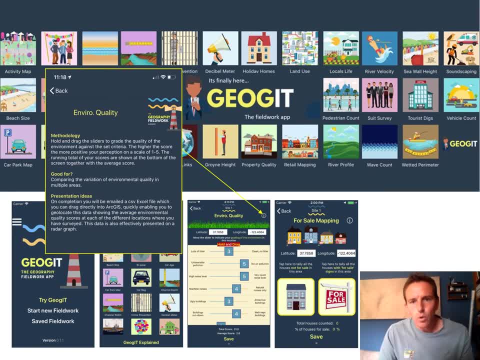 already got your data in an electronic format and, crucially as well, it's geolocated as well. so the coordinates of where you've taken your fieldwork is log2, which enables you to make GIS maps. so all of that sounds a bit technical. it is a little bit, I suppose, and so that's why. 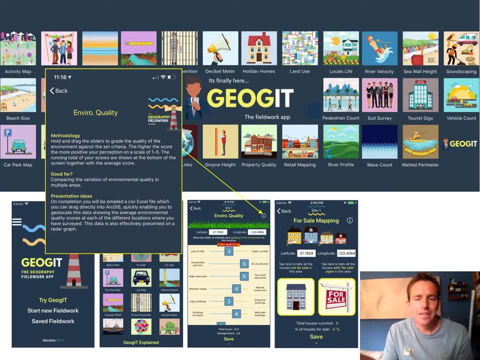 I'm going to do a kind of specific video on using technology to help with your NEAs and jog. it is one of those things I would absolutely recommend that you use and- but just at a glance at this stage- jog. it might well be something that's. 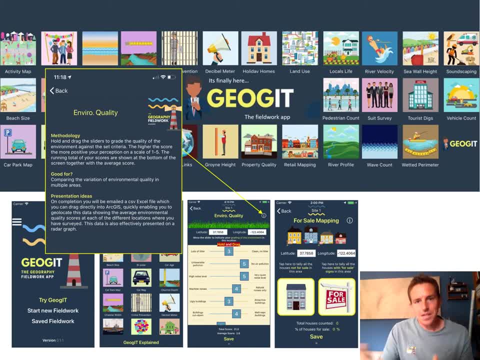 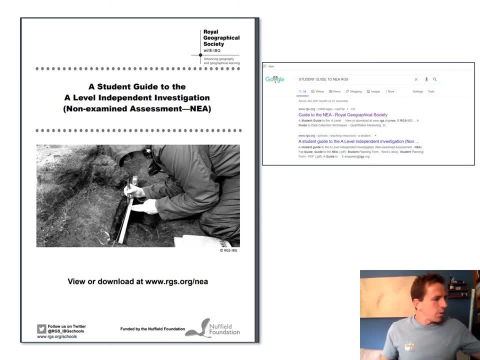 useful to have a look at to give you again an idea about some additional methods of data collection that you can use for your study. another thing at this stage which I think is worth me just documenting is this guide here. I've got my own copy here and I look after that. 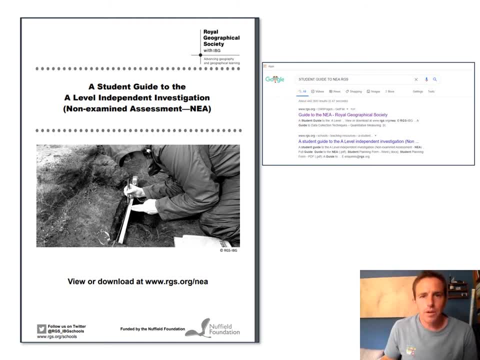 because it's it's excellent. this is something that was published by the Royal Geographical Society, I think, probably about a year and a half or so ago, and this is downloadable from Google and you can just see there or just screenshot what I typed into Google and this is the first result that you get up. 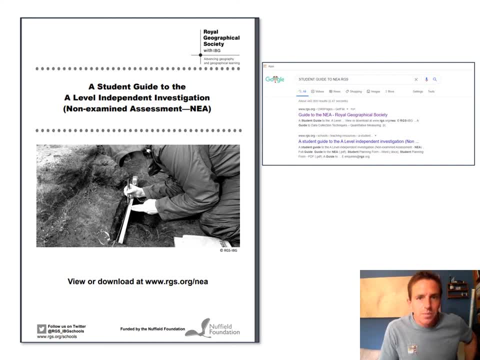 and it's a PDF. it's quite a hefty PDF- there's quite a lot of pages- and so maybe just save it somewhere where you can electronically access it rather than perhaps printing it off. but it has every different section that you would need to access for your NEA and but has lots of good ideas about different methods of 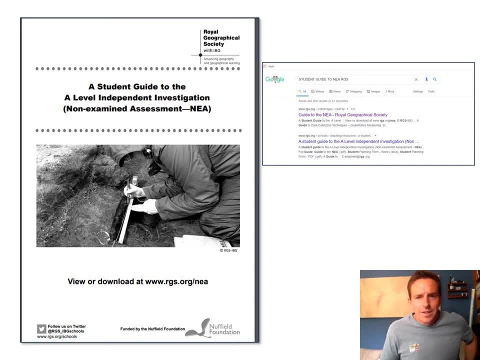 data collection, lots of ways in which you could present your data as well, and also really has good explanations about using stats tests in your NEA and when various stats tests might be suitable and supporting of what you're trying to do. so I would definitely recommend if 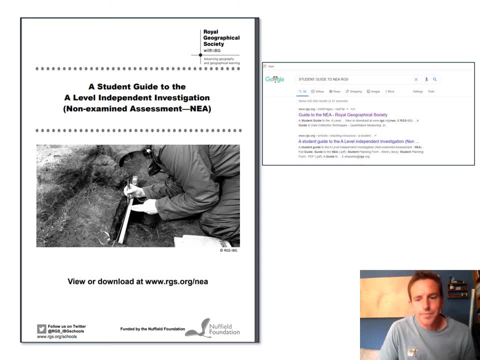 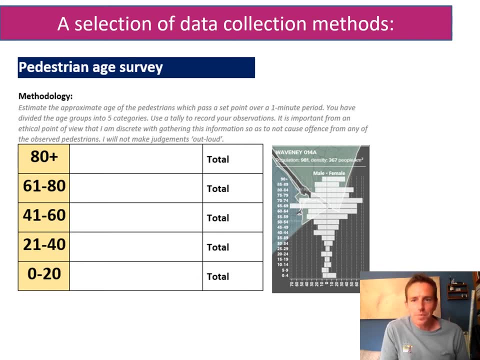 you haven't been told to. I'd recommend having a look at this guide. okay, so this session is really all about you choosing the methods of data collection which are going to be appropriate and relevant to your sub questions, and it's also about giving you some free time to think about how you would like to use the data collection. 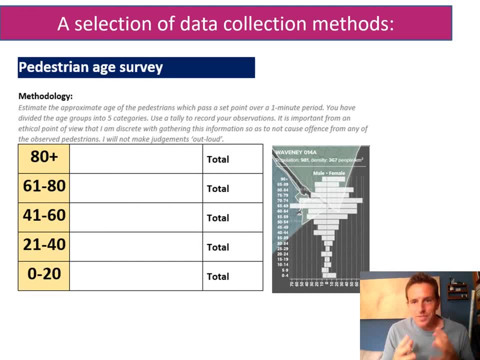 you a bit more awareness about the types of data and information that you can collect. now, what we're not going to do- because it would take us forever- is literally go through every single method of data collection that you can use, and also one of the things that we don't want to do is to kind of just force 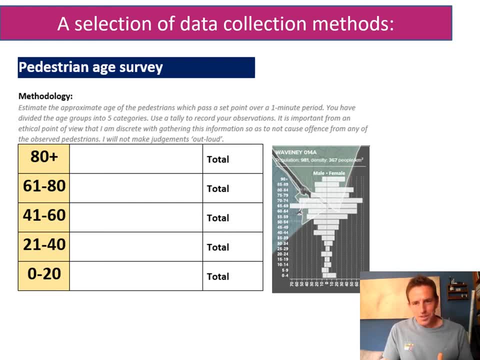 methods of data collection on you. it should be almost that you are thinking about the information that you need to gather and then you almost kind of design your own bespoke methods of data collection, and these ideas that we're about to go through could hopefully give you a little bit more of an idea. 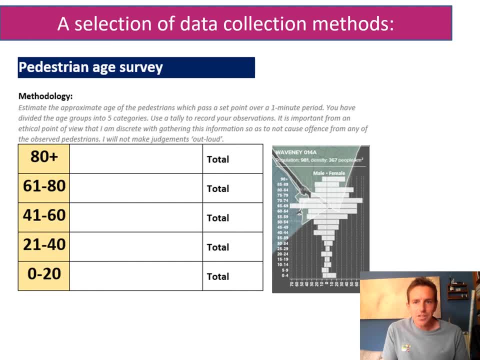 that actually, you can tweak established methods of data collection to suit your own study. you could perhaps change the scale and the spectrums and the words and maybe the sampling techniques that are being encouraged, and so one of the things that you need to think about with your fieldwork is that not only does 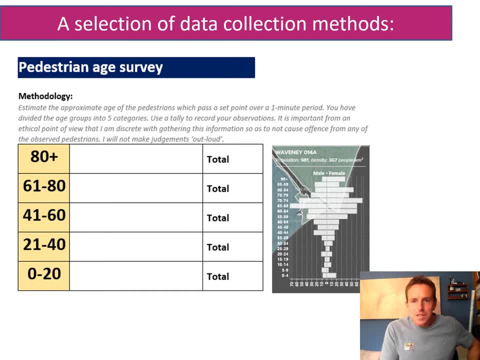 your title and the study need to be bespoke to you, but you should also think about the methods of data collection that you're using being bespoke to you as well, as the methods of data collection that you're using being bespoke to you as well and you put in your own angle on them and jog it is a fantastic tool for. 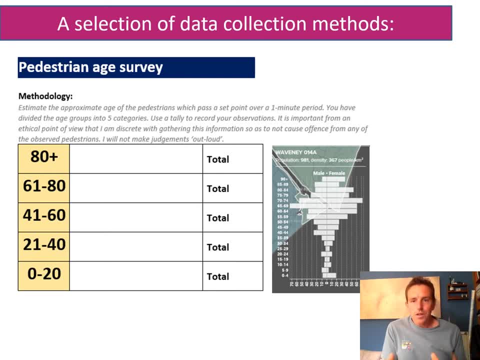 gathering data. but you might well look at some of those methods on jog it and think, actually I want to change that and I want to make that a little bit more unique to me. so there is an environmental quality survey, for instance, on jog it, but within jog it there are criteria already set amongst it and it's 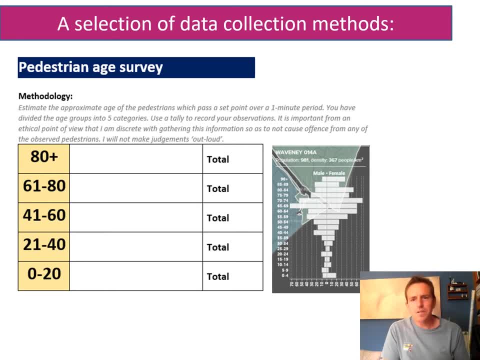 on a scale of one to five, those criteria. so you might well think: well, I want to do on the scale of one to ten and I'm not quite happy of the words that are being used in there. so I'm not quite happy with the words that are being used in there. 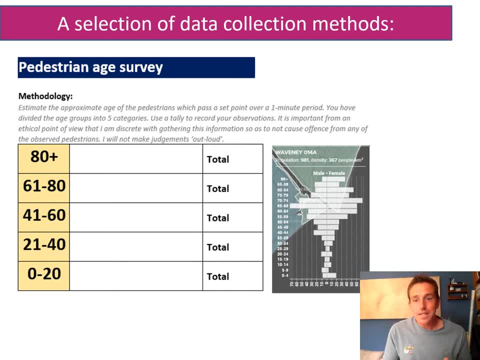 so that's fine. use it as a bit of an inspiration and as a bit of an idea. so that's fine. use it as a bit of an inspiration and as a bit of an idea about the types of things you can measure. but then do your own and come. 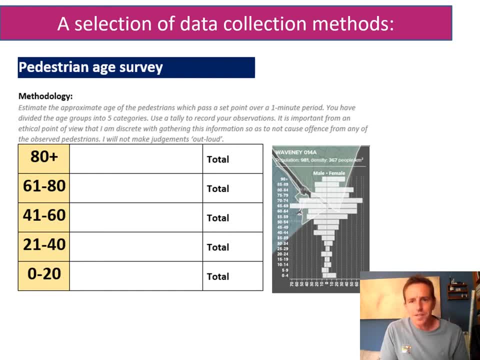 about the types of things you can measure. but then do your own and come out of your own spectrums and your own unique take on some of the surveys that. out of your own spectrums and your own unique take on some of the surveys that 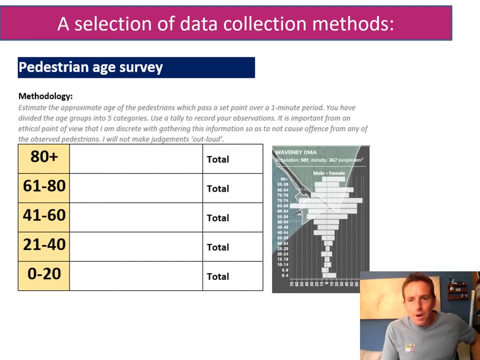 are out there for you to use, so with that in mind, I'm just going to start. are out there for you to use, so, with that in mind, I'm just going to start with this one here. I'm going to go through several more and the idea of me. 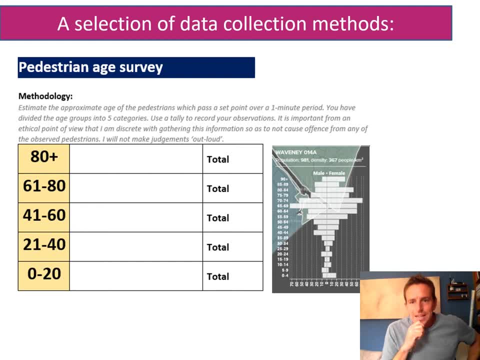 with this one here I'm going to go through several more, and the idea of me going through some of these selections of data collection methods is to kind of this one. here I'm going to go through several more, and the idea of me highlight some of the things that you could do to kind of make you was a 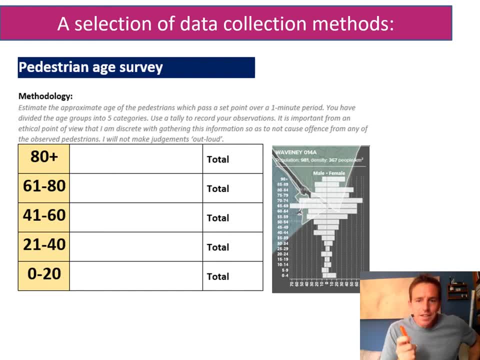 highlight some of the things that you could do to kind of make you was a little bit more bespoke. so one of the top five methods of data collection that little bit more bespoke. so one of the top five methods of data collection that we highlighted from our Twitter survey was a pedestrian count- now a pedestrian. 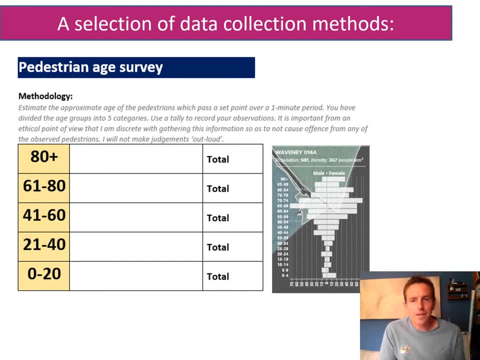 we highlighted from our Twitter survey was a pedestrian count. now, a pedestrian count is is fine, but it doesn't give you a huge amount of information. and one count is is fine, but it doesn't give you a huge amount of information. and one of the things that you could do is to kind of tweak and tailor a pedestrian. 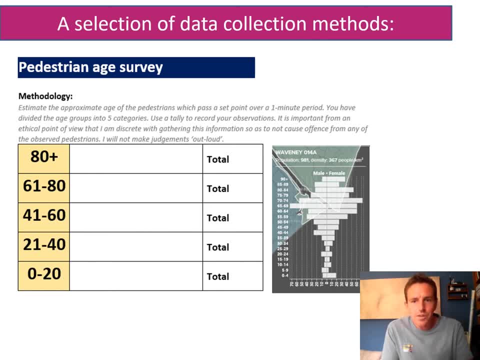 of the things that you could do is to kind of tweak and tailor a pedestrian count to make it more valuable. so if you were doing a study, for instance, on count to make it more valuable, so if you were doing a study, for instance, on something like identity and one of the things 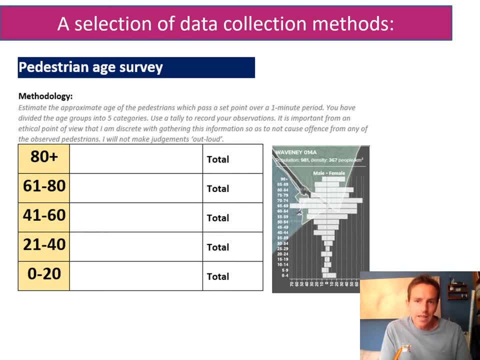 something like identity, and one of the things- something like identity and one of the things you could potentially try to do- is you could potentially try to do, is you could potentially try to do- is identify the age structure people in the. identify the age structure people in the. 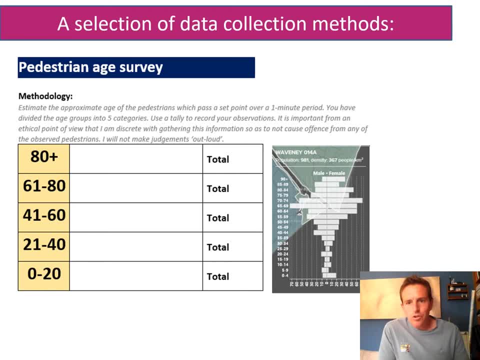 identify the age structure people in the location that you're investigating. so location that you're investigating, so location that you're investigating, so you could to try and gauge the ages of. you could to try and gauge the ages of. you could to try and gauge the ages of people in that location. you could go up. 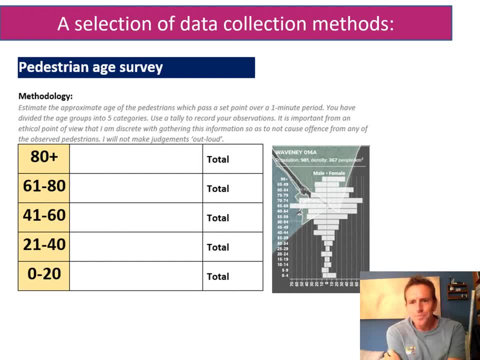 people in that location. you could go up people in that location. you could go up to them and say: excuse me, would you mind to them and say: excuse me, would you mind to them and say: excuse me, would you mind telling me how old you are? you might be. telling me how old you are. you might be a bit weird doing that, though, and they a bit weird doing that though, and they a bit weird doing that though, and they might think that that's a bit odd, and it might think that that's a bit odd, and it. 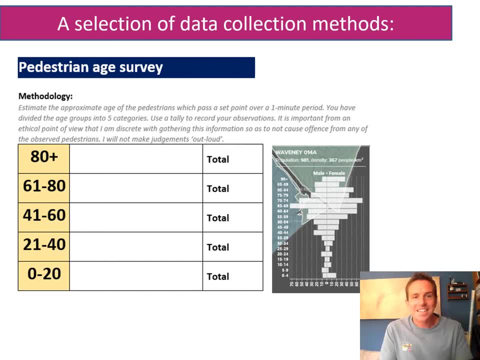 might think that that's a bit odd. and it is a bit odd, so I wouldn't do it. so what is a bit odd? so I wouldn't do it. so what is a bit odd? so I wouldn't do it. so what I would do instead is try to devise a. 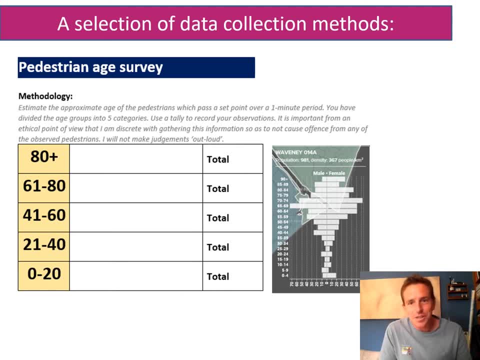 I would do instead is try to devise a. I would do instead is try to devise a way of discreetly doing that and you way of discreetly doing that and you way of discreetly doing that, and you could do this sitting down, which is. could do this sitting down, which is. 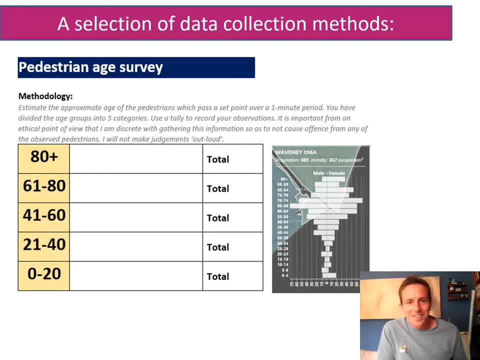 could do this sitting down, which is always nice. find a bench or somewhere- always nice. find a bench or somewhere- always nice. find a bench or somewhere you can sit in a location and, discreetly, you can sit in a location and, discreetly, you can sit in a location and discreetly make observations as to the age of. 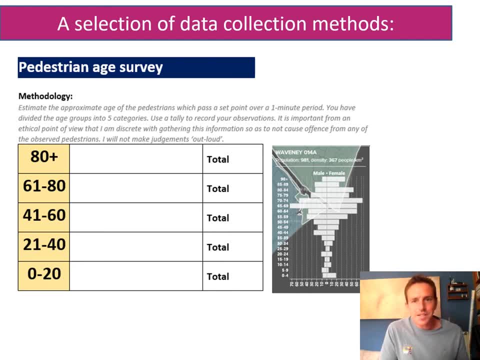 make observations as to the age of, make observations as to the age of people that you can see using that space, people that you can see using that space, people that you can see using that space. it might be that you do this as a time. it might be that you do this as a time. 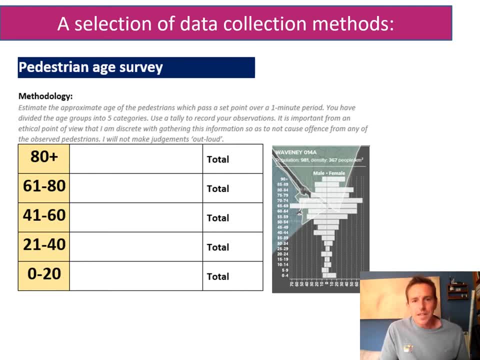 it might be that you do this as a time survey, perhaps over five minutes, and survey perhaps over five minutes, and survey perhaps over five minutes, and over five minutes, rather than just over five minutes, rather than just over five minutes, rather than just literally telling the people to give you. 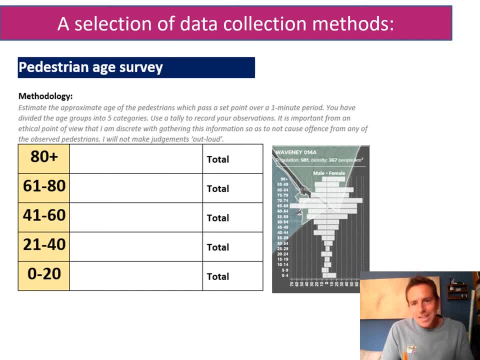 literally telling the people to give you, literally telling the people to give you a collective pedestrian count number. you a collective pedestrian count number, you a collective pedestrian count number. you could make that more useful by trying, could make that more useful by trying, could make that more useful by trying to allocate approximate ages to the people. 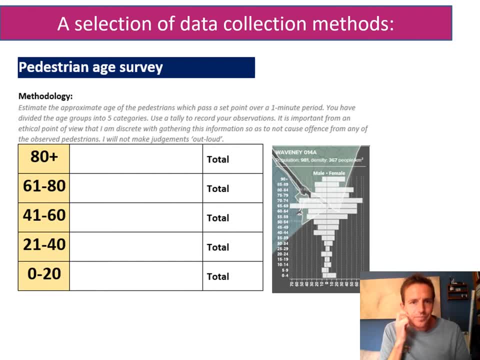 to allocate approximate ages to the people, to allocate approximate ages to the people that you can see in that location, as that you can see in that location, as that you can see in that location as well. so, on this scale, here we have. well, so, on this scale, here we have. 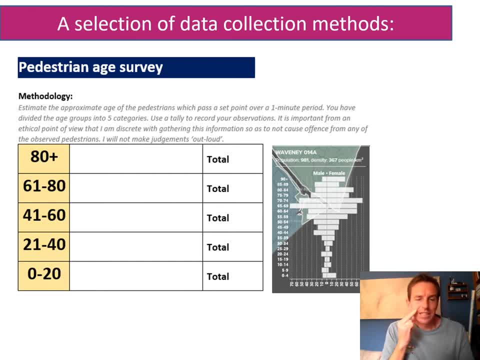 well, so on this scale, here we have divided people up into five categories, divided people up into five categories. divided people up into five categories: depressing, so you've got the youngsters. depressing, so you've got the youngsters. depressing, so you've got the youngsters between 0 and 20, you've got the young. 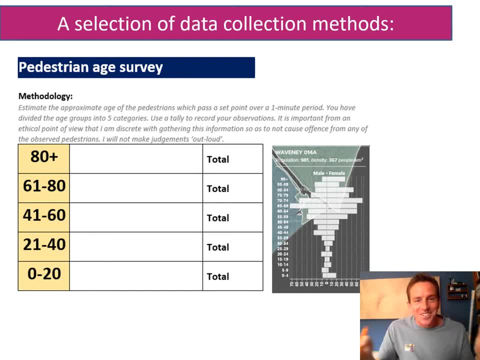 between 0 and 20. you've got the young between 0 and 20. you've got the young adults 21 to 40 above that. I don't know adults 21 to 40 above that. I don't know adults 21 to 40 above that. I don't know what you call that group. 41 to 60s and 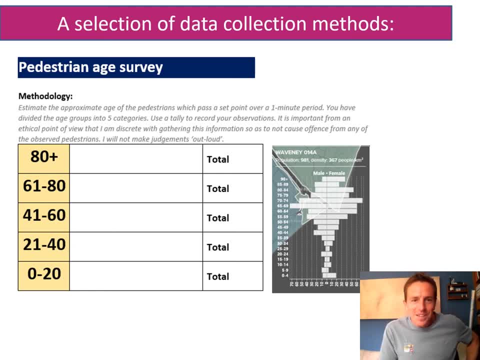 what you call that group 41 to 60s and what you call that group 41 to 60s, and then you've got 61 to 80 and you've got, then you've got 61 to 80 and you've got, then you've got 61 to 80 and you've got 80 plus. so we've decided for one of our 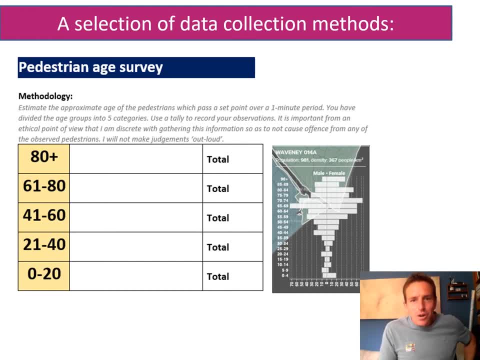 80 plus. so we've decided for one of our 80 plus. so we've decided for one of our key stage 3 studies to use this five key stage 3 studies, to use this five key stage 3 studies, to use this five start kind of step spectrum, because we 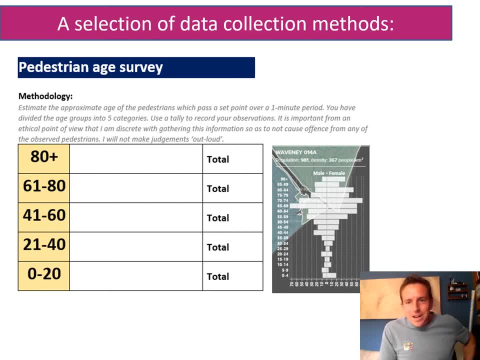 start kind of step spectrum. because we start kind of step spectrum because we felt that that was age brackets, that felt that that was age brackets, that felt that that was age brackets that were fairly easy to identify people in, were fairly easy to identify people in, were fairly easy to identify people in if you had kind of brackets of five. so 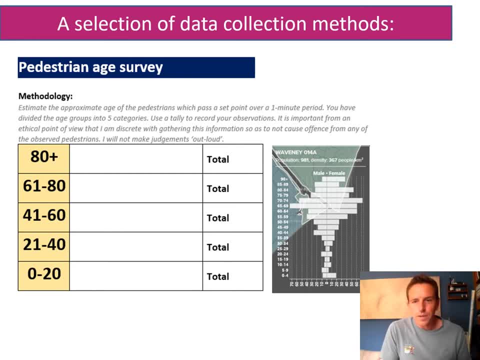 if you had kind of brackets of five. so if you had kind of brackets of five, so you had 0 to 5, 5 to 10, that would be you had 0 to 5, 5 to 10, that would be you had 0 to 5, 5 to 10. that would be fairly straightforward for getting. 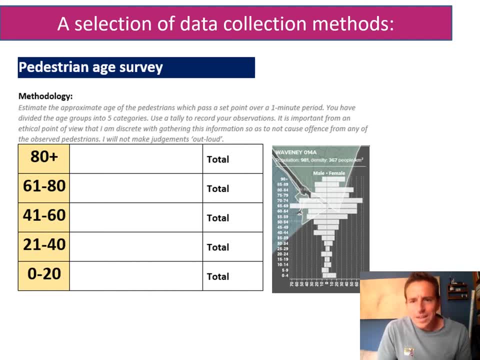 fairly straightforward for getting fairly straightforward, for getting people people's ages accurate. when people people's ages accurate. when people people's ages accurate when they're younger, but when people get into they're younger. but when people get into they're younger. but when people get into their 30s and 40s it's much more. 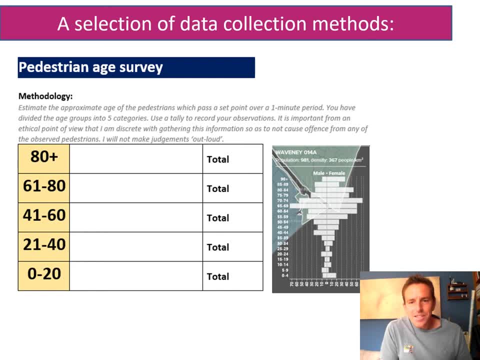 their 30s and 40s. it's much more their 30s and 40s. it's much more difficult for you to accurately, difficult for you to accurately difficult for you to accurately estimate somebody's age. I'll give you estimate somebody's age. I'll give you. 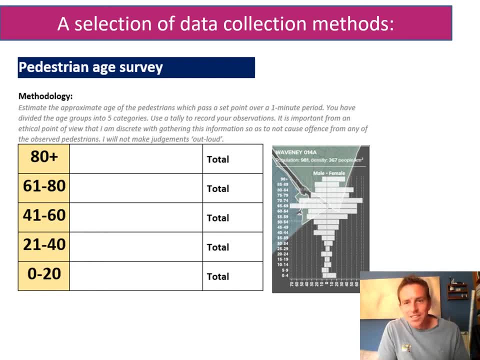 estimate somebody's age. I'll give you an example. can you estimate my age? if an example, can you estimate my age? if an example, can you estimate my age? if you said 23, you bang on, well done okay. you said 23, you bang on, well done okay. 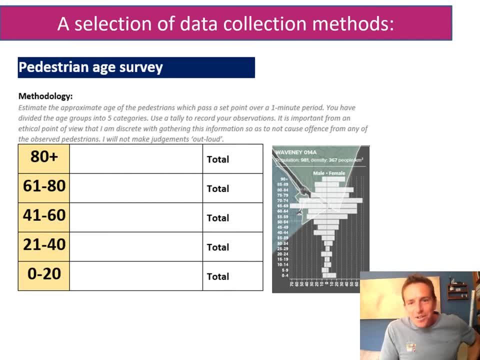 you said 23, you bang on. well done, okay. so this is a way in which you could. so this is a way in which you could. so this is a way in which you could potentially enhance a pedestrian count. potentially enhance a pedestrian count, potentially enhance a pedestrian count by turning it into a pedestrian age. 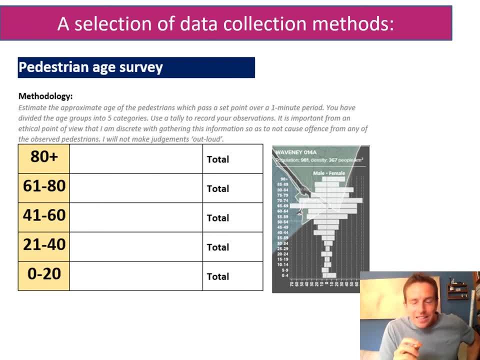 by turning it into a pedestrian age, by turning it into a pedestrian age survey, and what you might expect then is survey, and what you might expect then is survey, and what you might expect then is that the results that you get would fit, that the results that you get would fit. 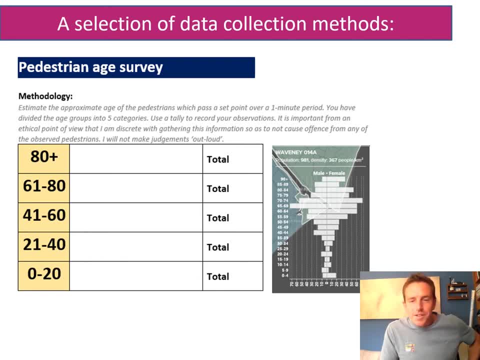 that the results that you get would fit with the population pyramid for that, with the population pyramid for that, with the population pyramid for that location and, as I mentioned on a location, and as I mentioned on a location, and as I mentioned on a previous session, parallelcouk is a. 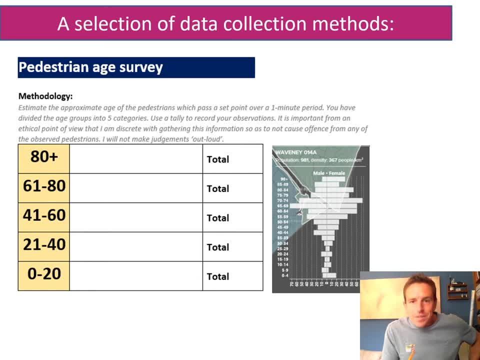 previous session. parallelcouk is a previous session. parallelcouk is a fantastic website that you can visit and fantastic website that you can visit and fantastic website that you can visit and you can get a pedestrian count and you can get a pedestrian count and you can get a pedestrian count and- sorry, a population pyramid for every. sorry, a population pyramid for every, sorry, a population pyramid for every single location, and that's what we've, single location, and that's what we've, single location, and that's what we've got there on the right-hand side of the got there on the right-hand side of the. 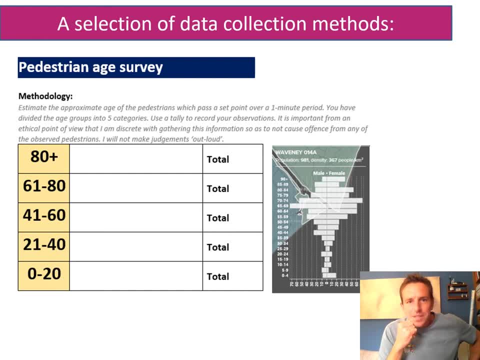 got there on the right-hand side of the screen and therefore we would expect screen and therefore we would expect screen and therefore we would expect that when we're doing a pedestrian age, that when we're doing a pedestrian age, that when we're doing a pedestrian age survey, that it would correlate with the. 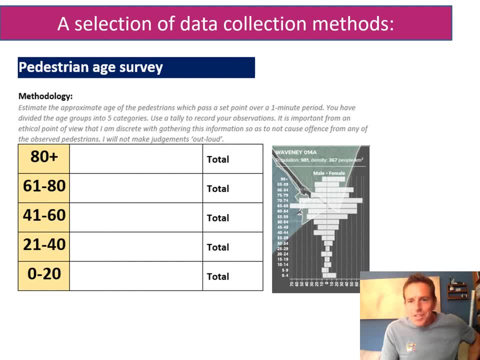 survey, that it would correlate with the survey, that it would correlate with the population pyramid for that location. so population pyramid for that location, so population pyramid for that location. so there are a number of limitations to. there are a number of limitations to. there are a number of limitations to this and actually one of the things that 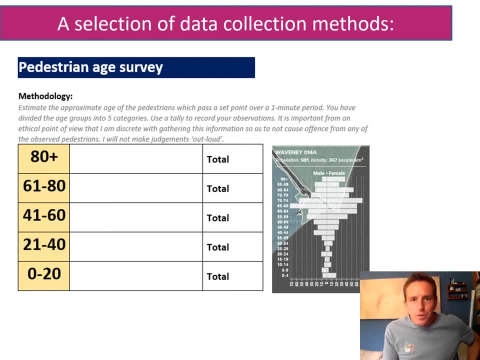 this and actually one of the things that this and actually one of the things that is quite useful to get in the mindset of, is quite useful to get in the mindset of, is quite useful to get in the mindset of early on when you're doing fieldwork, is 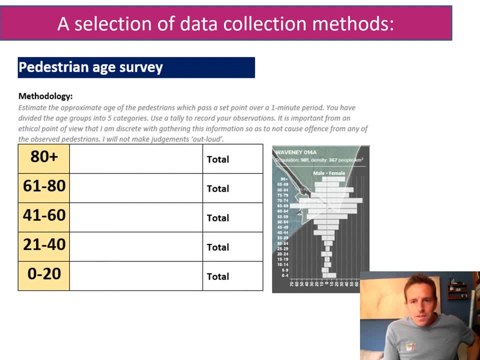 early on when you're doing fieldwork is early on when you're doing fieldwork is having limitations and weaknesses to having limitations and weaknesses to having limitations and weaknesses to methods is not a problem. the problem is methods is not a problem. the problem is methods is not a problem. the problem is where you try to pretend that there. 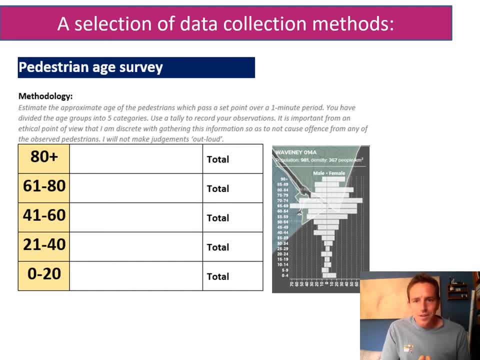 where you try to pretend that there, where you try to pretend that there aren't weaknesses and limitations to aren't weaknesses and limitations to aren't weaknesses and limitations to methods, and actually it's a quite a good methods and actually it's a quite a good methods and actually it's a quite a good thing to have limitations, because that. 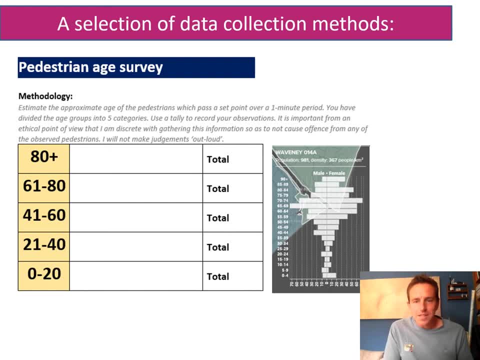 thing to have limitations, because that thing to have limitations, because that then gives you quite a lot of things to then gives you quite a lot of things to then gives you quite a lot of things to talk about in terms of reliability of talk about, in terms of reliability of. 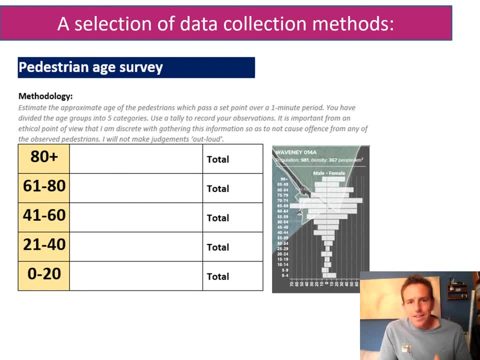 talk about in terms of reliability of your data and as long as you can say your data, and as long as you can say your data and as long as you can say that you know, you're aware that this is, that you know, you're aware that this is. 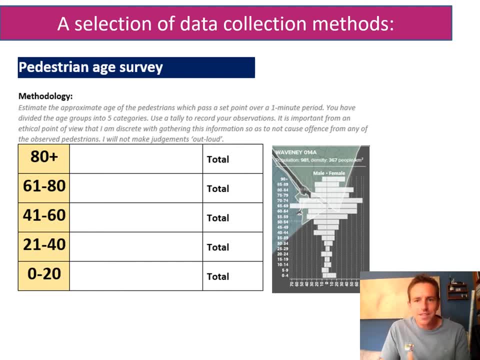 that you know, you're aware that this is this method of data collection, isn't this method of data collection? isn't this method of data collection isn't necessarily the strongest and these are necessarily the strongest and these are necessarily the strongest and these are some of the limitations of it, and that's. 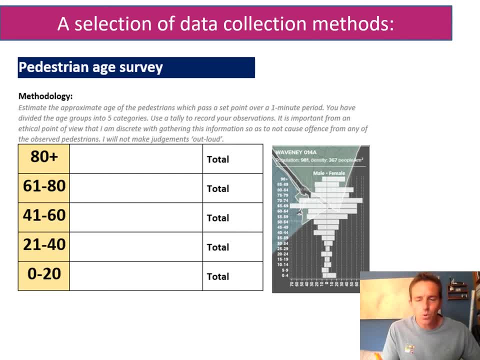 some of the limitations of it. and that's some of the limitations of it, and that's fine because it isn't expected that. fine because it isn't expected that. fine, because it isn't expected that your fieldwork should be black and white. your fieldwork should be black and white. 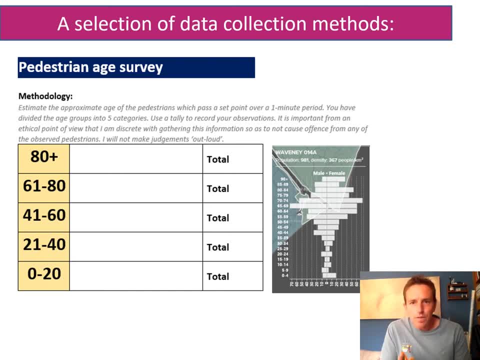 your fieldwork should be black and white, watertight, scientifically accurate and watertight, scientifically accurate and watertight, scientifically accurate and for a lot of human methods of data, for a lot of human methods of data, for a lot of human methods of data collection especially, they can be quite 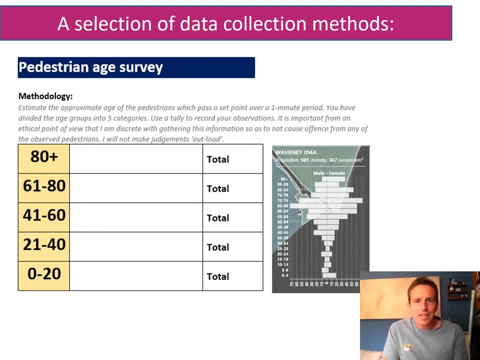 collection, especially they can be quite collection, especially they can be quite vague and they might not necessarily be vague and they might not necessarily be vague and they might not necessarily be scientifically black-and-white accurate, scientifically black-and-white accurate. scientifically black-and-white accurate, hundred percent reliable. but having an 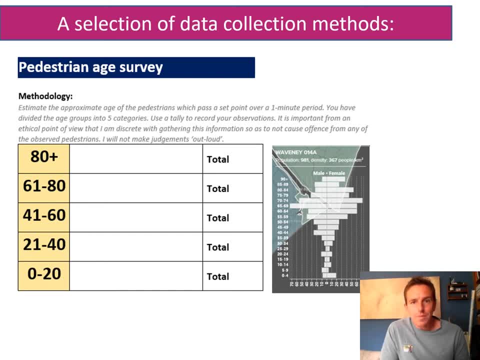 hundred percent reliable. but having an hundred percent reliable, but having an awareness that they're not reliable is awareness that they're not reliable, is awareness that they're not reliable is the key thing. and talking about the, the key thing, and talking about the, the key thing and talking about the limitations and weaknesses of them is 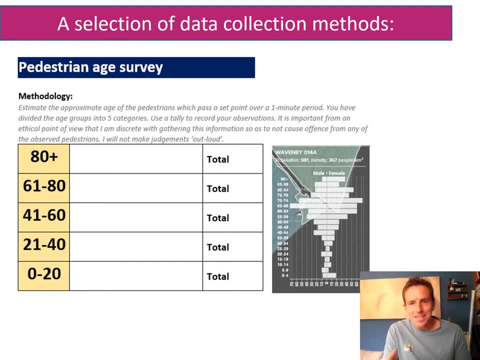 limitations and weaknesses of them is limitations and weaknesses of them is the important thing that you do so, the important thing that you do so, the important thing that you do so. pedestrian age survey has definitely got. pedestrian age survey has definitely got. pedestrian age survey has definitely got weaknesses. it's definitely not. 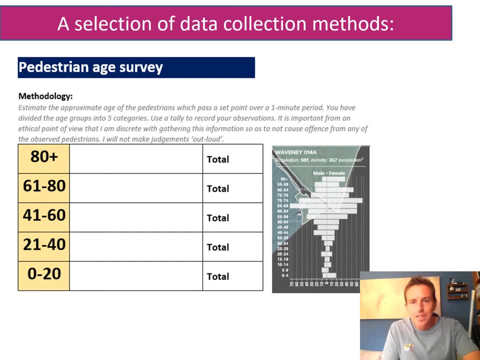 weaknesses. it's definitely not weaknesses. it's definitely not bulletproof, but you can still use it as bulletproof. but you can still use it as bulletproof, but you can still use it as long as you're aware of the weaknesses, long as you're aware of the weaknesses. 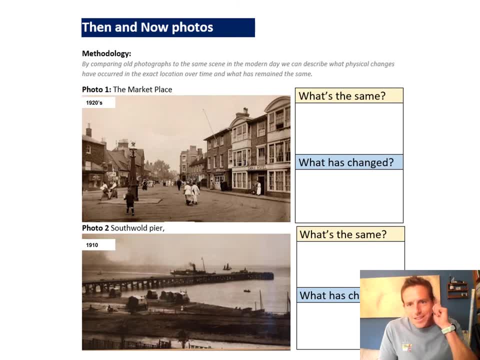 long as you're aware of the weaknesses of it, and this one is a really easy nice of it, and this one is a really easy nice of it, and this one is a really easy nice thing to do then and now photos, and I thing to do then and now photos, and I. 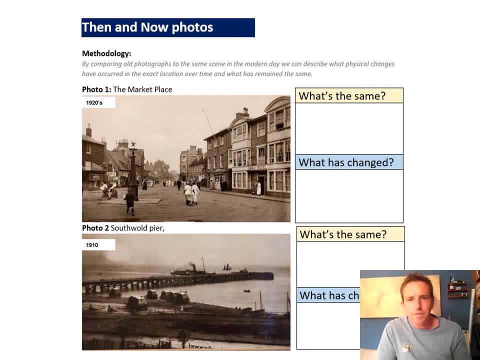 thing to do then and now photos- and I think it's a second on the list and think it's a second on the list and think it's a second on the list- and photographs and field sketches and using photographs and field sketches and using photographs and field sketches and using photographs and field sketches is a. 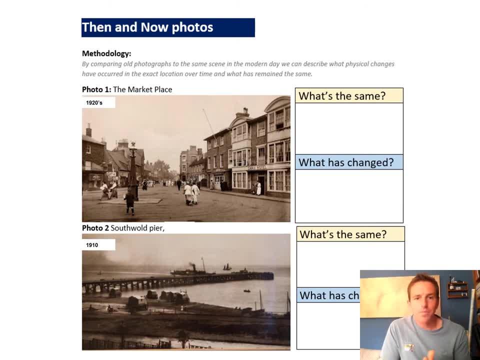 photographs and field sketches is a. photographs and field sketches is a great way of looking at change over time, great way of looking at change over time, great way of looking at change over time and how things have perhaps changed, how and how things have perhaps changed, how and how things have perhaps changed, how identities might have changed, and one: 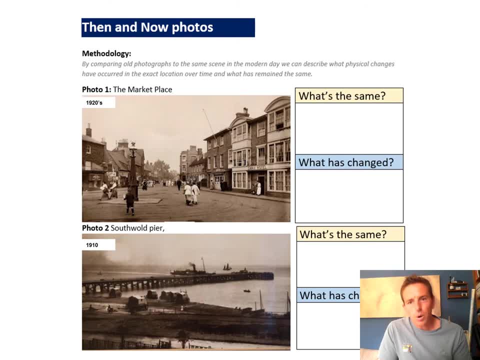 identities might have changed and one identities might have changed and one of the things that you can very easily do, of the things that you can very easily do, of the things that you can very easily do on Google and probably lots of other on Google and probably lots of other. 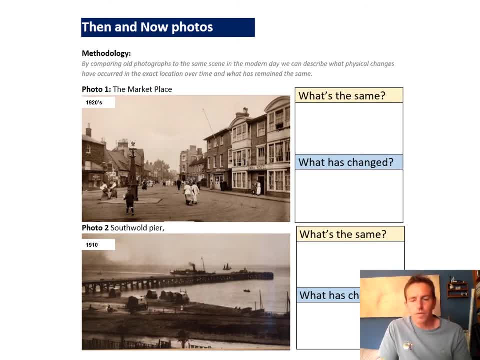 on Google and probably lots of other websites, is find historic pictures of the websites. is find historic pictures of the websites. is find historic pictures of the places that you're investigating and places that you're investigating and places that you're investigating, and try and get a selection of these and then 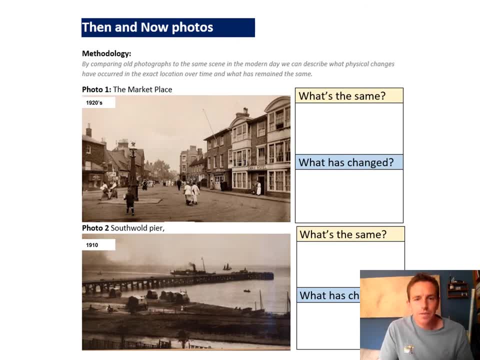 try and get a selection of these, and then try and get a selection of these, and then try and replicate the exact view in, try and replicate the exact view in, try and replicate the exact view in the modern day, and if you can, then compare the modern day and if you can, then compare. 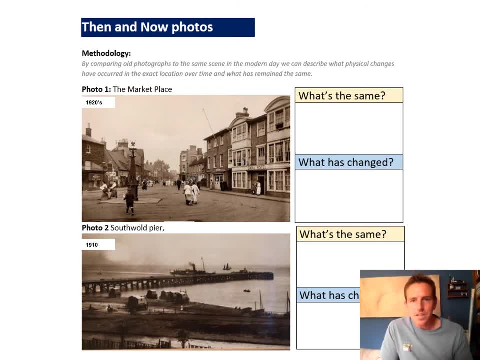 the modern day and if you can then compare that view side-by-side of the past, that view side-by-side of the past, that view side-by-side of the past and present view, you can look at and present view. you can look at and present view. you can look at physically how the area has changed and 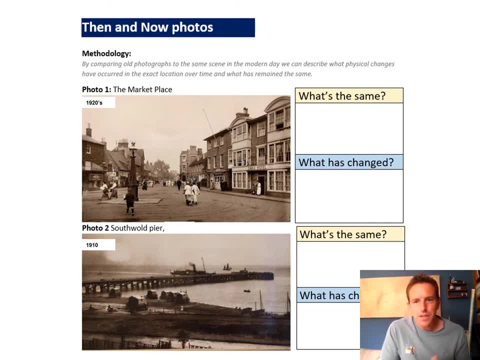 physically how the area has changed and physically how the area has changed and what things have remained the same and what things have remained the same and what things have remained the same, and it's a very nice kind of visual way. it's a very nice kind of visual way. 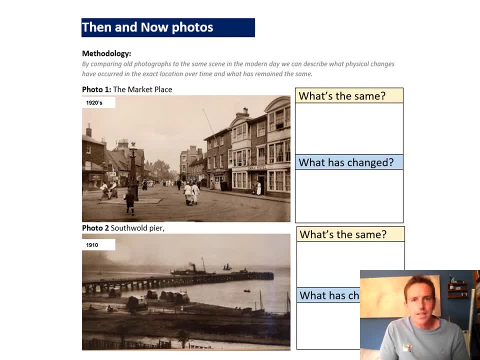 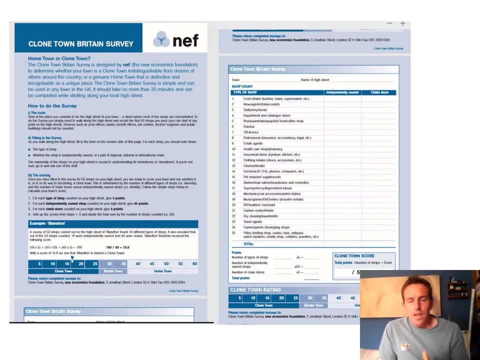 it's a very nice kind of visual way, particularly in the early stages, perhaps, particularly in the early stages, perhaps, perhaps of your NEA, to look at the change over time, if that's one of the things that your study is focusing on. Quite a few teachers got back to me and said that- one of the things that they do. 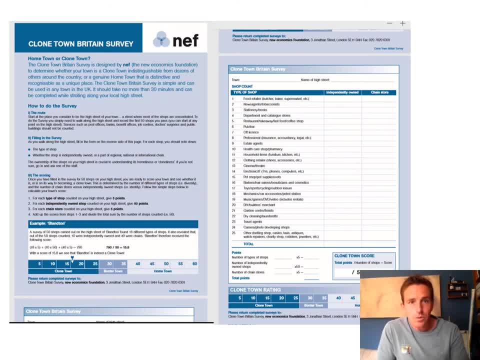 with their Key Stage 3 students with a local town study is this thing called a clone town survey, and this isn't one of the methods that we have got on Joggett because it's slightly more complex, but it's a really useful thing to look at. Again, if you google clone town survey, this, I think, is 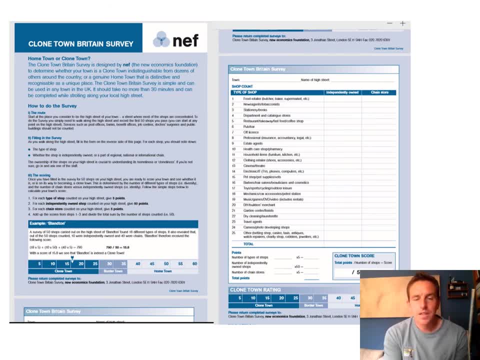 the first result that comes up, and it's a pdf that you can download and on one side it has a kind of a table that you fill in and on the other side it has the step-by-step guide as to how to complete a clone town survey. Ultimately, it will give you a score having done this kind of. 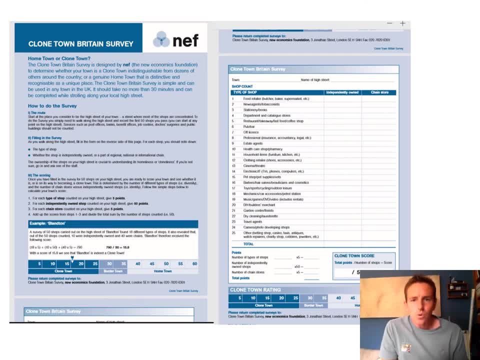 fieldwork method. you'll get a score, And that score will tell you how unique that town is, or that town's high street is, in comparison to other towns in the country. Now it might well be that you are able to access historical data to show what your high street was like historically. So in South Old, for instance, in Suffolk, where we're 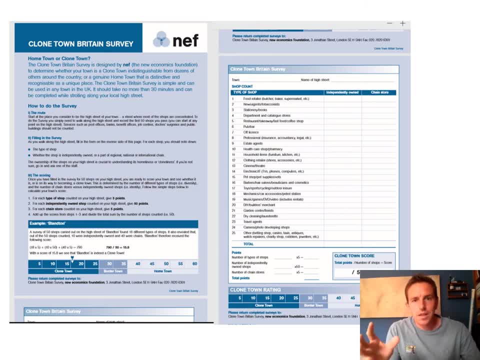 based. we have a fantastic website which allows us to look at the use of every single commercial building in the town, dating back to about 150 years. So actually we've been able to produce clone town surveys for our high street, not just in 2020, but in 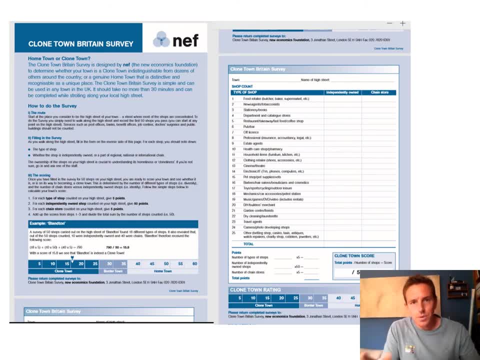 2010,, 2000,, 1990, any year in fact, we could do a clone town survey of. So we can see how, over time, South Old High Street has become more of a clone to other high streets in the country, because it 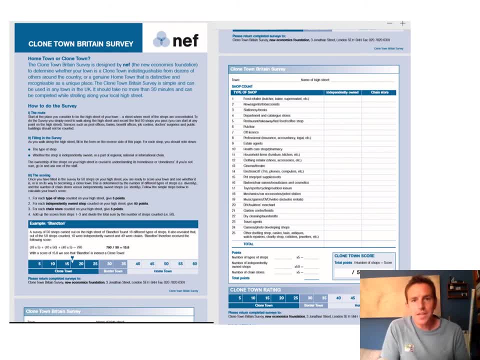 has seen an increasing rise in chain stores coming into the high street. So a clone town survey is brilliant and if you can do some digging, some secondary research, it may help you a little bit. It may well be possible that you can do a clone town survey not just for 2020, but over time as well. 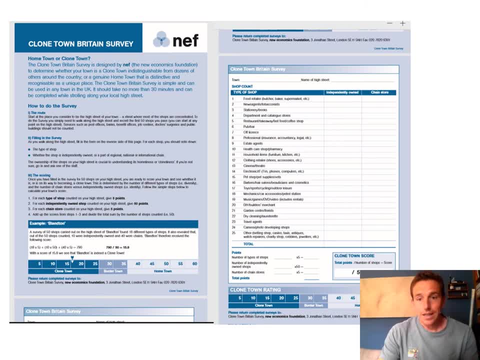 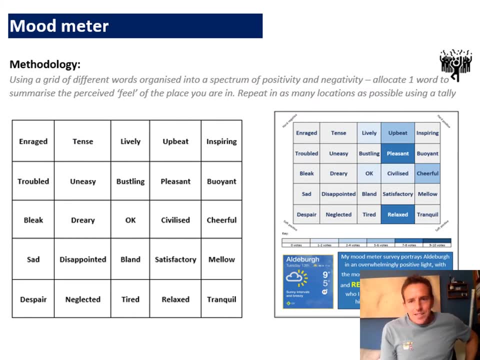 So that's one that perhaps would help you looking at how, again, identity and change over time has impacted your area. The mood meter is something which has actually been developed from a theory which has been, I think, developed by an American psychologist, and they came out of this idea that 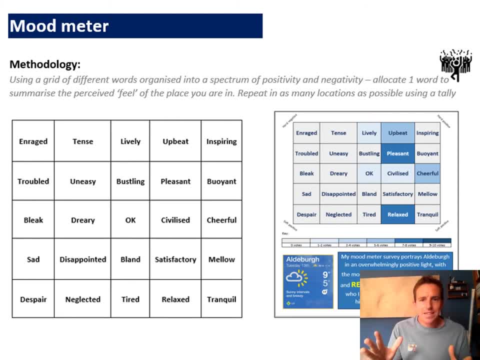 there is a spectrum of words that can be allocated from the most negative to the most positive, and any given place, whether it's indoors or outdoors, can have an atmosphere to it or a mood associated with it. So, for instance, this room that I'm currently in, at the moment, is excited and, you know, enthused, and hopefully your 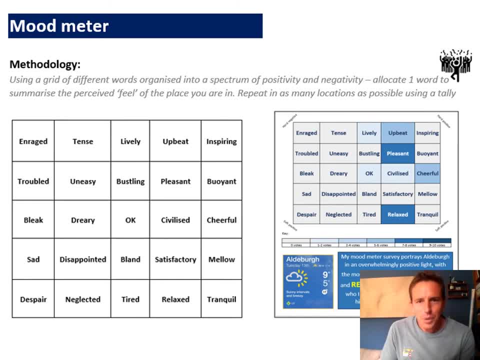 room that you're watching this in is also bustling, inspired, buoyant and just eager to get out there and complete field work. Now, if you look at the grid that you've got there on your screen, select the word now that you are actually feeling. Hopefully, you're not feeling sad or bleak. 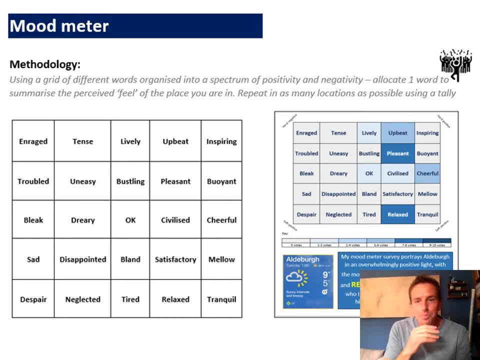 but you're feeling cheerful, maybe buoyant, upbeat. So that's the same with a space, whether it's indoors or outdoors. If you're going to a town or a city or a beach, that area will have an atmosphere that you can give to it, and this is something that planners are. 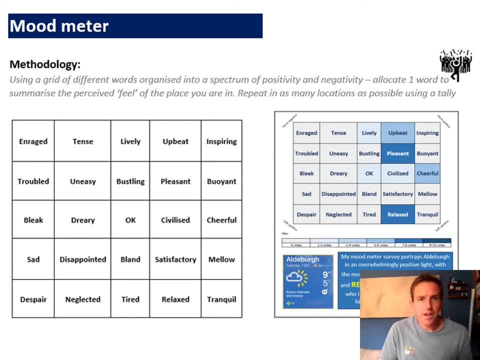 aware of and they try, when they're creating regeneration projects or redevelopment projects, to not only create successful commercial and residential spaces, but to also create a pleasant atmosphere in places that encourage people to be there and aren't hostile or negative in any way. So one of the things that you can try and do to assess the identity and the success of 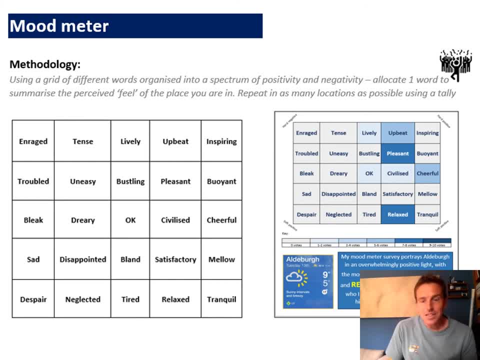 regeneration or, you know, the identity of places is to actually consider the mood of that place. And again, I've spoken earlier about things being slightly vague and not necessarily hugely scientific. Well, this is kind of as wishy-washy as it gets, but that doesn't necessarily mean you. 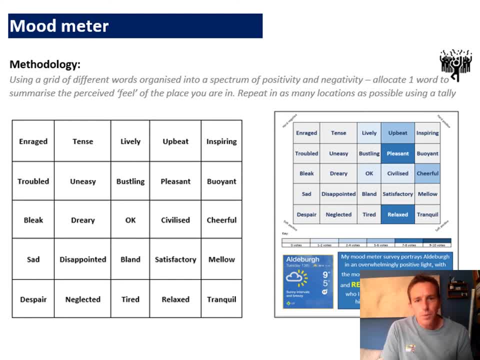 shouldn't do it. A mood meter can be made more reliable if you give other people the opportunity to contribute to the survey that you're doing. If you just went to a high street and said, stood there, closed your eyes for a second and just took it all in and said, yeah, I reckon this is okay and that. 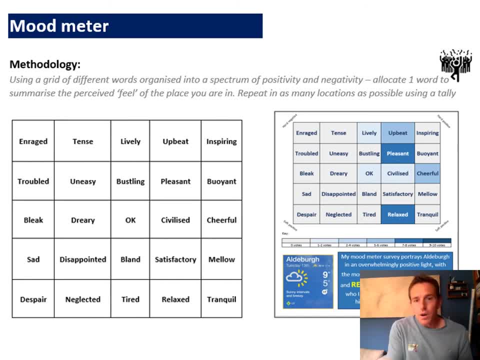 then was your result, then that's pretty much it. So if you're going to a high street and you're going to be in a place that's really limited, but if you asked 100 people, if you said to them: look, I've got this scale here, would you mind just thinking and telling me which word on this scale? 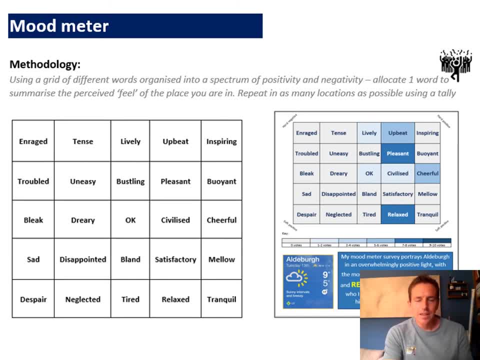 you think best fits the atmosphere of this place currently. and if you've got 100 of those responses, then all of a sudden that becomes much more valid, much more useful in your study. So again, the mood meter is something that is on Jogit, but on Jogit we have this set of words. It might well be that 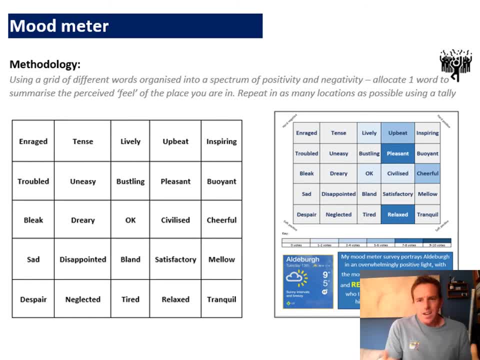 you take inspiration from that and you say, okay, I quite like that idea, but I'm going to make this a bit more bespoke to me and I'm going to make my own spectrum. I'm actually going to have 50 words and these are going to be my words. and on: 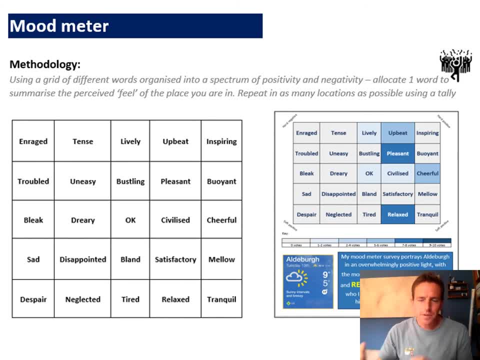 the top right hand side are going to be the ones that are most positive. on the bottom left hand side are going to be the ones that are most negative. What you potentially could then do is to perhaps have that grid laminated. it doesn't have to be laminated, but it's nice if it is. 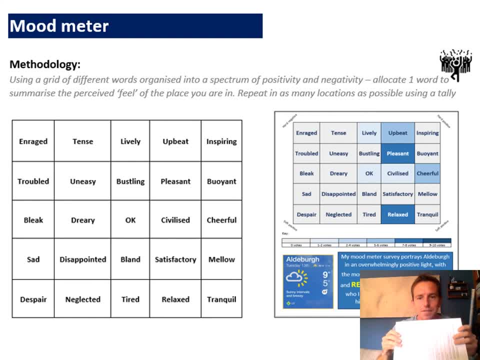 and you could then perhaps say to people on the street from a safe distance: would you mind just kind of saying which word on this scale would fit the atmosphere of this place? So if you've got 100 words on this grid best fits the atmosphere that you think this place represents, You might think 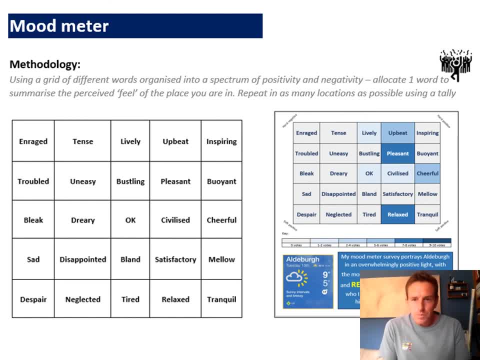 about other ways in which you could perhaps get people to contribute to that without physically actually speaking to them. So it might be that you create an online survey and you have 10 pictures of the town that you're investigating or the location that you're investigating. 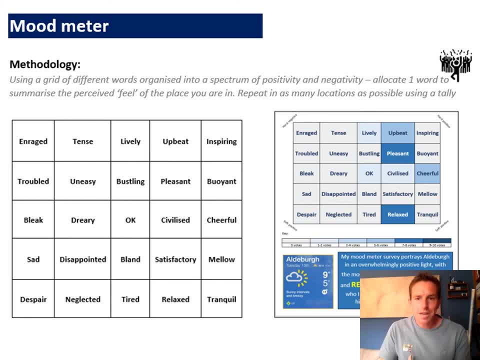 and you let people see those 10 pictures and at the end of those 10 picture slideshow, for instance, you then give them this grid and you say, having seen those pictures of this town, what were the words you think perhaps best fits the mood that has been created in this environment? and they could. 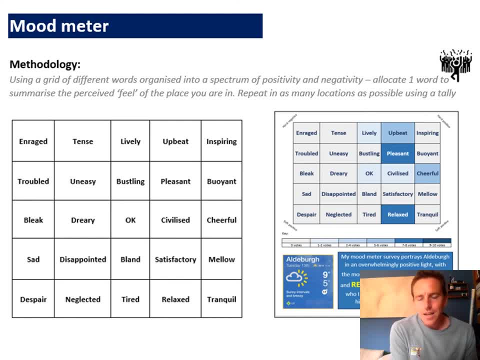 then just select the word from your list. So a mood meter is again a different way of collecting qualitative opinion based data and it can be made much more useful and much more valid if you get more people to contribute to that survey. You can just see on a screen above my head that one of the 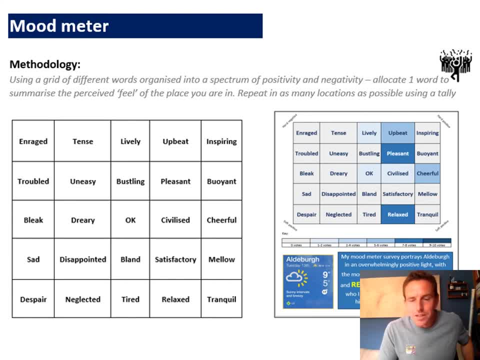 other things that you might need to consider with some of the methods of data collection that you do, are the external factors beyond your control that will influence the reliability of the results that you get. So, for instance, when you're doing coastal studies, if you're doing things like longshore drift, 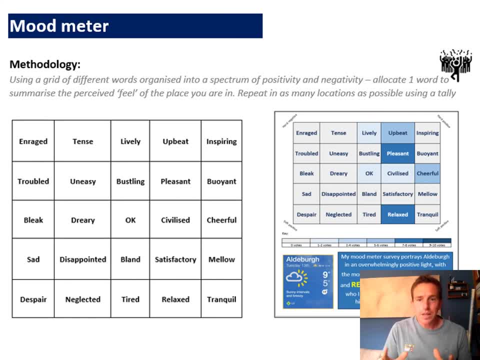 measurements. one of the factors that's beyond your control and that will influence your results is the strength of the wind and the strength of the waves, and also the state of the tide on the time, on the days and the times on those days that you're measuring your results. 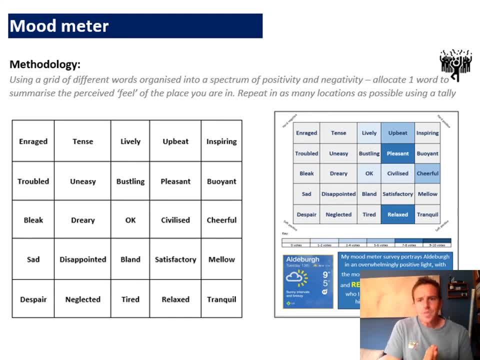 With something like a mood meter. if you're asking people to give you a judgment as to what their opinion is on the mood or atmosphere of a place, one of the things inevitably that will give them a kind of a something to factor into or influence their opinions will be the weather. 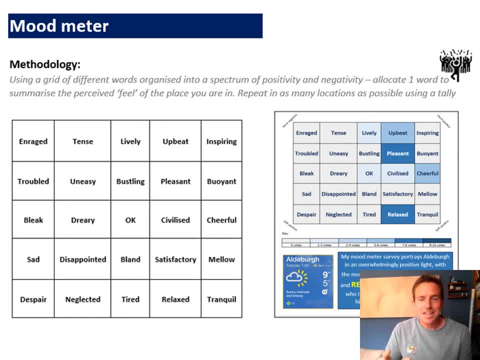 on the day, and if it's a very nice, hot, sunny day, people are generally going to feel much more positive about the place. if it's pouring of rain again, that's going to have a negative impact. Might well be as well that you know. you have people saying things more negatively at the moment because of the weather. 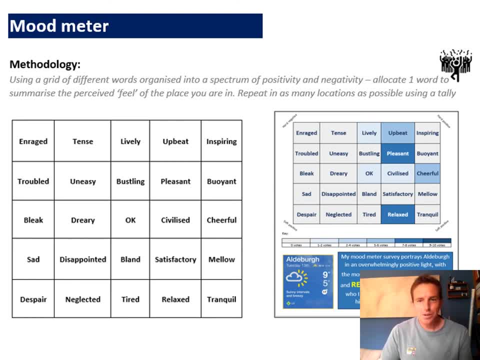 The current situation with the coronavirus. so that is an external factor beyond your control. So these are the kind of small details that actually show that you're really thinking about the validity and the reliability of the data that you're collecting, and I would suggest that, as they're coming into your head, you should make a note of those, because 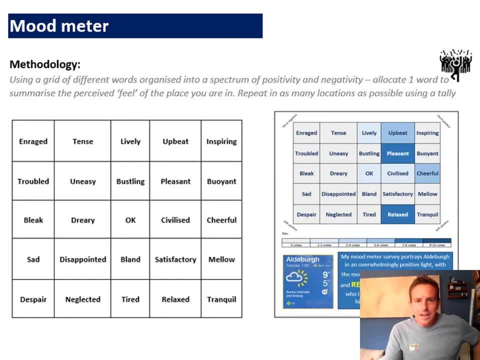 when it comes to your evaluations, when you're talking about how good your data is- which is what your field work is kind of really trying to encourage you to do is to reflect on how good your data is- Then the more kind of things that you can say like that that actually the accuracy was impacted by this or the 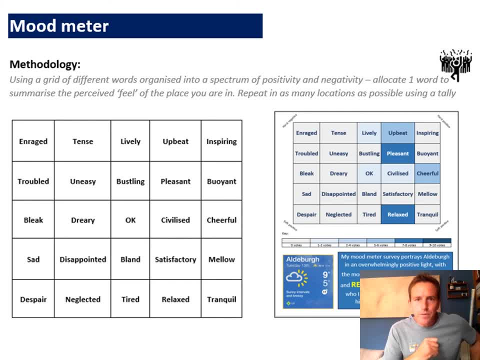 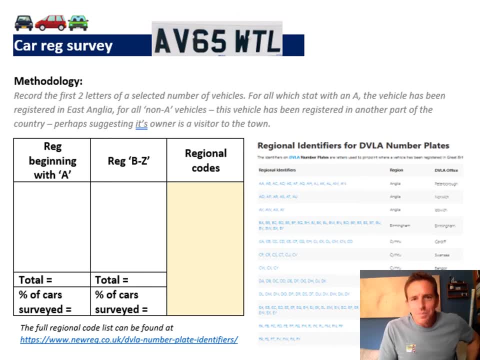 reliability might have been impacted by this, then you'll get more credit for it. So a mood meter is a good way of kind of highlighting some of those issues. Okay, so this is quite a nice method to consider, and the reason I've included this one is that 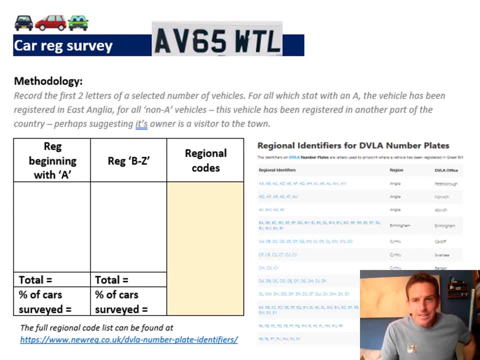 there are a number of things that you can do just by looking at vehicles that give you an indication about ownership and the identity of people in a particular place and also success of particular place, depending on number of vehicles. But there's quite a lot of car surveys that you can do at a safe distance without actually having to. 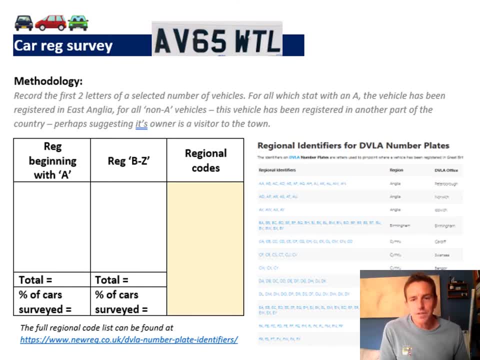 physically speak to people. Just make sure, obviously, if you're doing any kind of car based survey, that that vehicle's not moving and there's nobody in it, because if you're standing with a clipboard or a phone and you're kind of making details about a vehicle, you don't 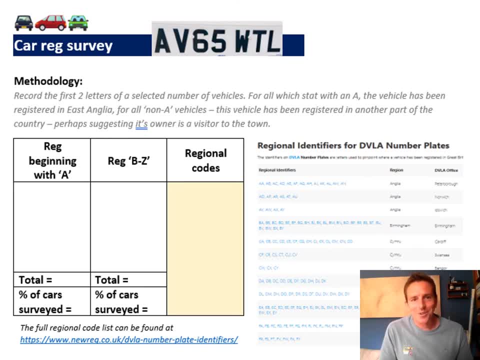 want to get into a confrontation with the person that's driving it or who owns it. Now, this method here is something called a car reg survey. Now, you may or may not know that all cars have a registration plate on the front of them. I'm sure you know that. 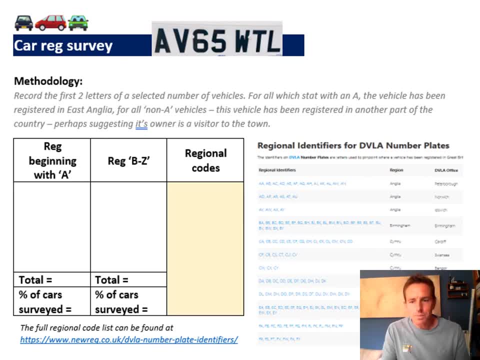 and as unless those cars have got personalised registration plates, then you can actually get quite a bit of information from the numbers and the letters that are on that number plate. So the first two letters relate to where that vehicle has been registered and where it was first purchased. So this one here has got AV. Now any vehicle that starts with the letter A. 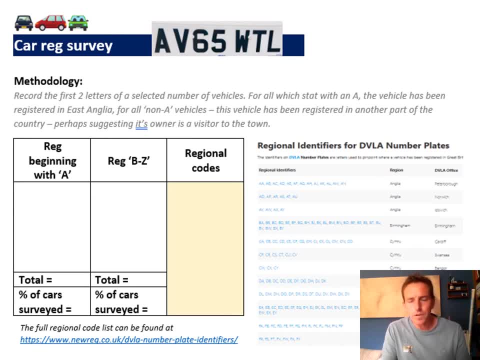 has been first registered in the Anglian region of Norfolk and Suffolk. So we know that in Southwold any vehicles in and around our town that have got an A registration plate are likely to be driven by local people. And it's much more likely that they are local people if that vehicle is newer as well. So the 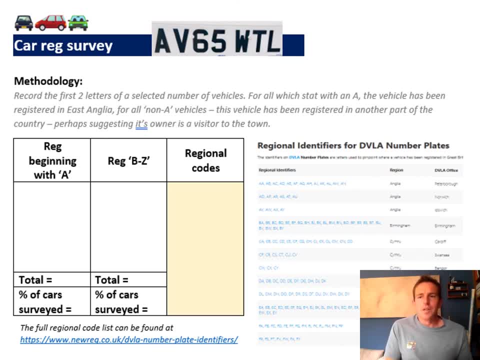 more new a vehicle is, the more new it still belongs to the original owner, the person who first registered it. Now you can get an idea about how new the vehicle is by looking at the numbers on a registration plate. So those numbers correlate with the year in which the vehicle was registered. So, for instance, 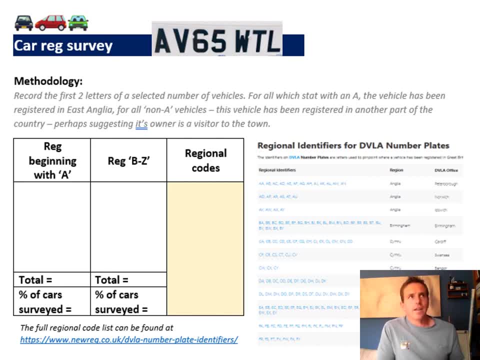 an 05 registration plate is 2005 and I think the latest one. what would that be? 19 or 20, I think it must be 20. now are the latest ones, but I'm not sure this year if those registrations have been released. That's probably a question for somebody else. 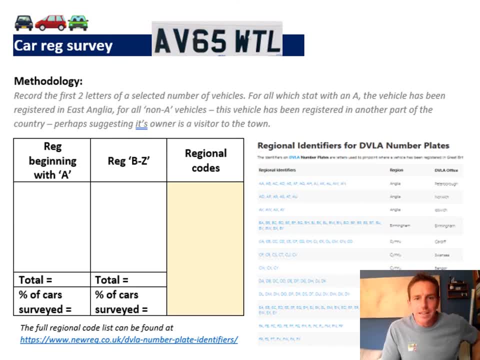 But the numbers on a registration plate will tell you how old that vehicle is. So we use this then to look at, potentially, where people have come from to visit Southwold, our town, And we say to students that, okay, if you just base this on vehicles that are three years old and less. 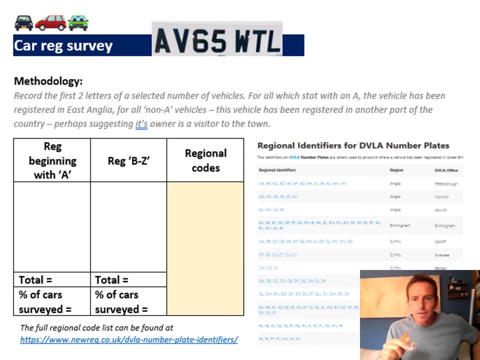 so three, two or one year old vehicles, and you look at the first two numbers, first two letters of the registration plate, and just take those numbers. you can then work out what proportion of vehicles are likely to be driven by local people and what. 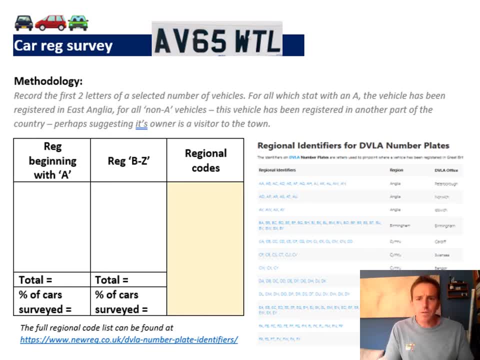 proportion of vehicles are likely to be driven by people who've come from further afield. So in our location we have a huge amount of second homeowners and that influences the identity and the demographic makeup of the town And one of the way and ways in which we can try to 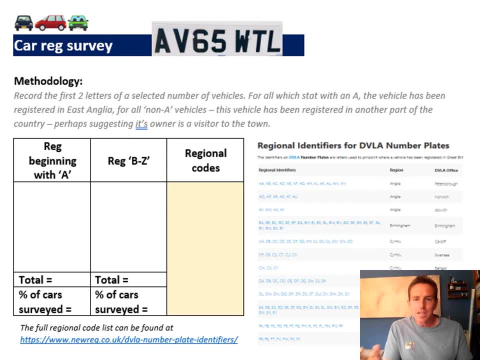 measure the extent of second homeowners and holiday makers is by looking at the registration plates of the vehicles in the town. Might well be that you're looking at the sphere of influence for a particular facility in your local area or a high street and using the car registration plates. 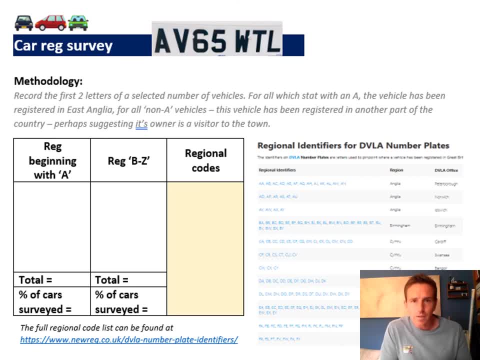 might be useful for that as well. 19- 00.01.190.075. thing that you can think of with vehicles is maybe just actually looking at the type of vehicle that you've got so to make and the model, the year, and if you go on something like AutoTrader and you type in those details and make the 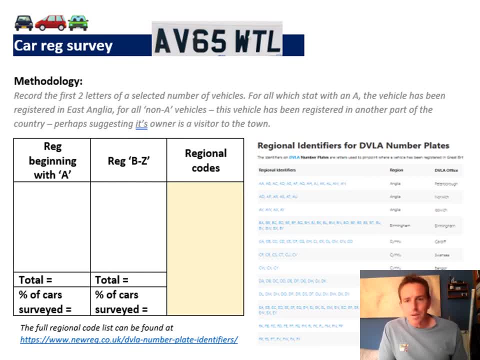 model and the year of a vehicle. obviously you haven't got the mileage of it, but you will be able to have enough criteria to get an idea about how much those vehicles are valued at. so it might be that you take the details of 50 vehicles, for instance, and you write those down from one location and you 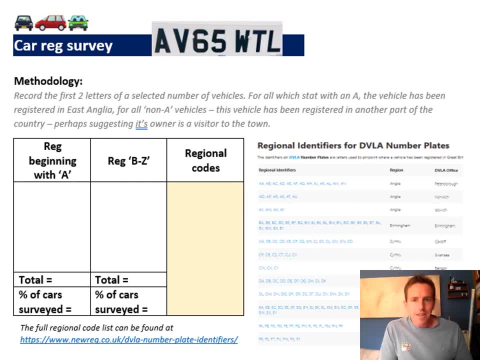 compare that to 50 vehicles in another location, and you might then be able to go on to AutoTrader to get an overall average as to how much the vehicles in one location are valued at in comparison to how much the vehicles in the second location are valued at- to get an idea, perhaps, of how wealth varies between two. 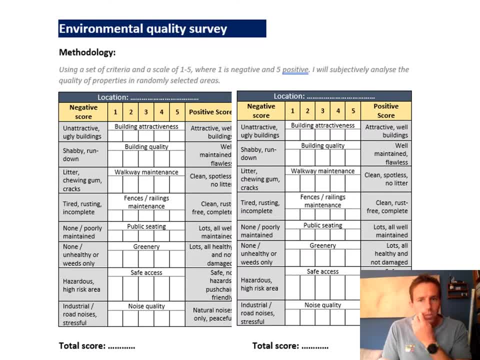 different places, so this one was voted number one of the all-time geography fieldwork methods- which is the one that I'm going to show you in a moment- which are being completed in high schools between years 7 and 11: the environmental quality survey. the reason that I've put it here is that 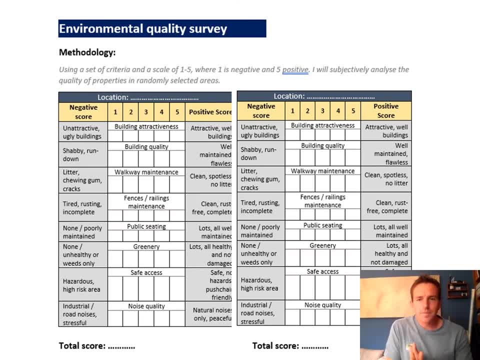 environmental quality survey is a template for basically any kind of qualitative survey that you want to do, and it's a really useful, really useful method. so we have taken this format and used it for a huge amount of different surveys: property quality survey, a residential quality survey, it can be. 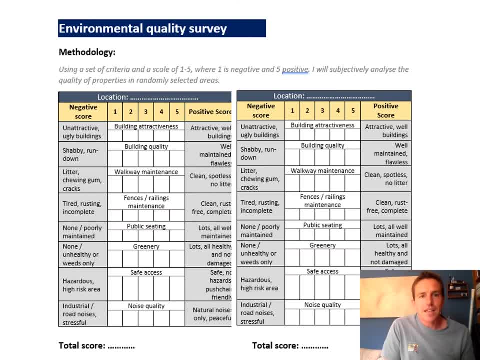 anything. the idea is that if you want to do a quality survey, you need to have a. an idea of this kind of grid is that you can come up with your own spectrums, your own scales and your own criteria. so down one hand side or the left hand side in. 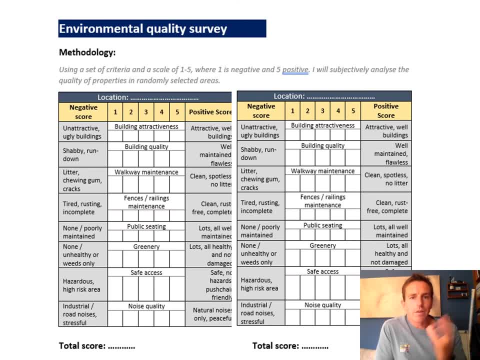 this instance, we've got the negative criteria and then on the right hand side we've got a positive criteria and then in the middle between the two we have the spectrum, and on this instance it's looking at a spectrum of 1 to 5. now you 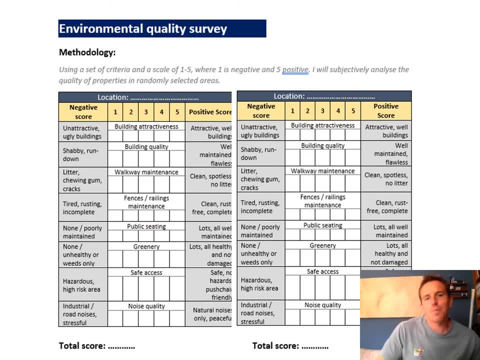 can make your own quality surveys by coming up with your own criteria and and your own spectrums, and this is something that i'd suggest you do. with the environmental quality survey, again, this is generally fairly kind of subjective if you're only going to be using it yourself. so if you're going to be doing these surveys yourself, then that's fine, but that 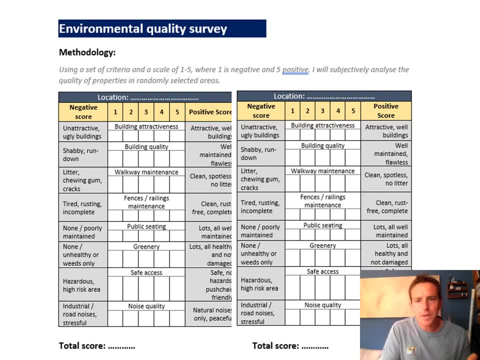 means the reliability of your data is a little bit limited to your own opinion, so you could make these perhaps more valid by asking, in different locations, other people to contribute to the environmental quality as well, and so, ultimately, what you can do with the environmental quality survey is gain a total score, and that total score then can be compared from one location to the. 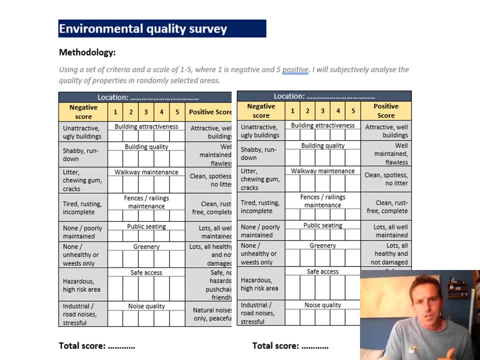 other. as i say, we use the same structure to do a property quality survey and we can do that then on different streets around the town. what we do when we're in those streets is we get the latitude and longitude coordinates of those locations and we make a note of those, and then that enables us at a later date to create a gis, a kind of an arc. 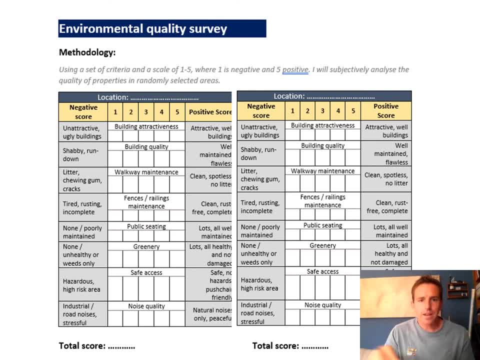 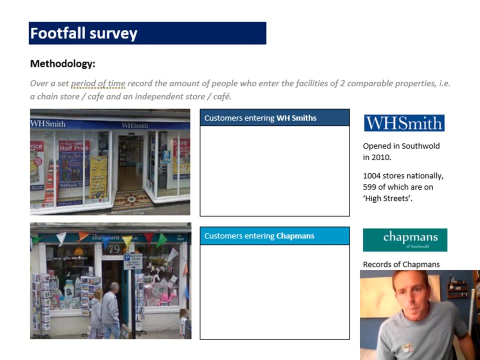 gis map that has got the variety, the varying environmental quality scores mapped out depending on where they were located from and where they were gathered from. so you can be very creative with this and you can make it bespoke to you. this one footfall survey is probably. 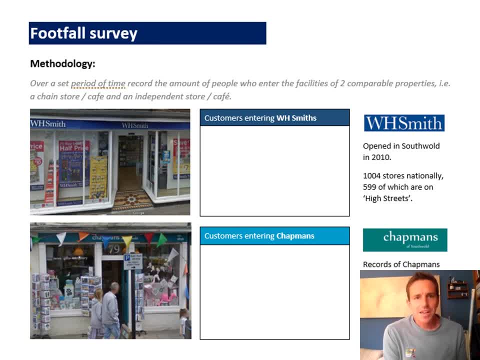 slightly incorrectly placed within this presentation and it perhaps could be more relevantly placed next to the pedestrian age survey, because this, ultimately, is another way in which you could tweak a pedestrian count rather than just randomly counting people. try and do it with some purpose and some function. 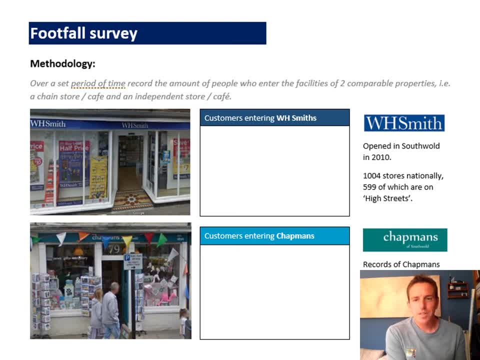 so for this one, a footfall survey is where you perhaps try to compare the amount of people visiting the different facilities and shops within a high street, and looking at footfall gives you a, you know, a useful way of comparing the success of one thing in relation to another. so, on our high 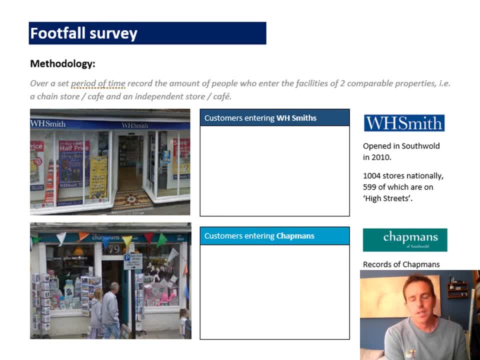 street in south world. we have a number of independent stores, but we also have a number, an increasing number, of chain stores. so we have this shop called chapman's, which has been run by a local couple for a long time, but it's the only chapmans in the whole country and it's 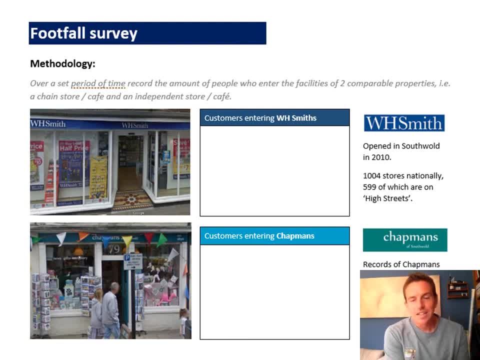 very much a kind of a unique, independent, very nice newspaper or news agents selling magazines and cards, bits of straight stationery and things like that. um 10 years ago in south world we had wh smith arrive for the first time and they- most of you- have been in wh smith's, you know what they sell. 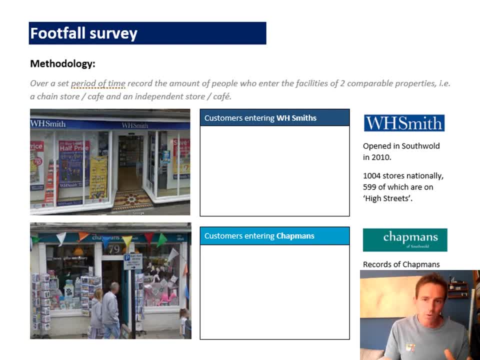 but they were in direct competition with chapmans and unfortunately almost directly opposite them, on different sides of the road as well. so a number of people, particularly newcomers into south world, knew about wh smith's and were probably drawn to wh smith's because they are familiar with it, whereas 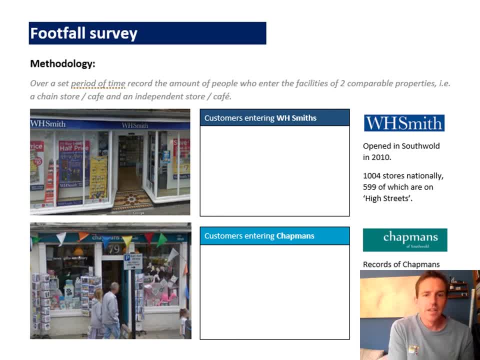 other people are perhaps more keen to support the independent store and support chapman. so one of the things that's changing in south world over time is that we're seeing an increasing amount of chain stores and we're seeing a decreasing amount of independent stores. so if that was one of the issues, 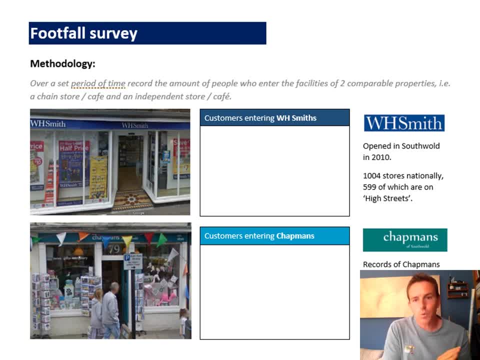 that you might want to focus your study on, then actually doing a footfall survey to get evidence of whether more people are supporting chain stores rather than independent stores would be a nice thing to do, so you could stand for five or ten minutes outside the front of these facilities. 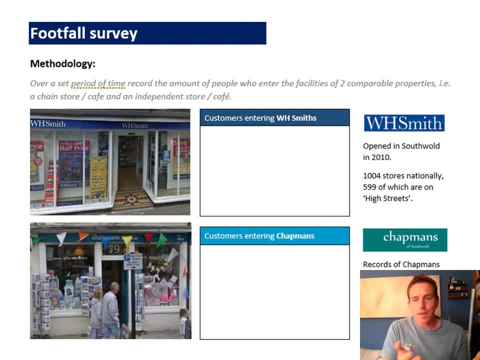 in these shops and you could literally make a survey, or a survey which enables you to tally the amount of people that are going in these stores during that time. again, you might need to think about how you would increase the reliability of doing this, and would you need to repeat this survey more than once? i'd 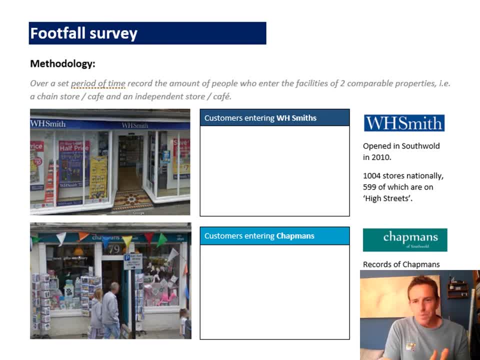 suggest that, yes, you probably would. you might need to repeat it over different days as well, just so you don't get any kind of anomalies. one of the ways in which you could tweak this as well is you could maybe perhaps do a shopping bag exit survey. so yes, people might be going into chapman's, but are they spending money? 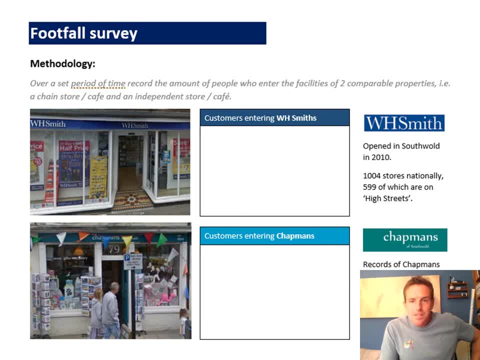 in chapman's, are people then going into wh smith's and spending money in wh smith's? so one of the things you could look at again discreetly is how many people are emerging from these shops actually carrying things that they've bought, whether they're in shopping bags or whether it's obvious. 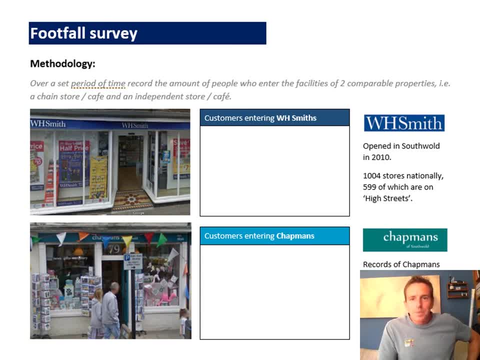 that they're carrying a newspaper or a magazine. so it might well be, again, that you're discreetly able to make a judgment about the trade that these stores are doing by doing a shopping bag exit survey. that is literally a method of data collection that i've just come up with- and that is what i'm saying- that you could. 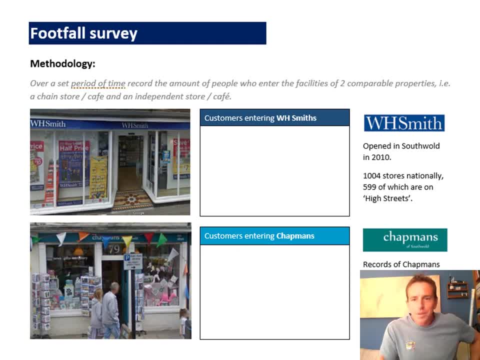 perhaps try to try to do, try to make up some of your own methods of data collection, having got inspiration from other, more established methods of data collection that already exist, like the classic pedestrian count. how could you tweak that pedestrian count to make it more relevant to the study that you're actually ultimately choosing? 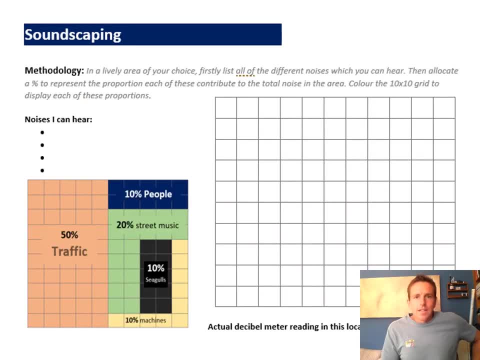 to do. okay, soundscaping: um, i mentioned earlier that mood meet, the mood meter was a little bit vague and a little bit wishy-washy. well, actually this is a different level. um, soundscaping is where you could. if you wanted to. you could go into a location. you kind of close your eyes, get at one. 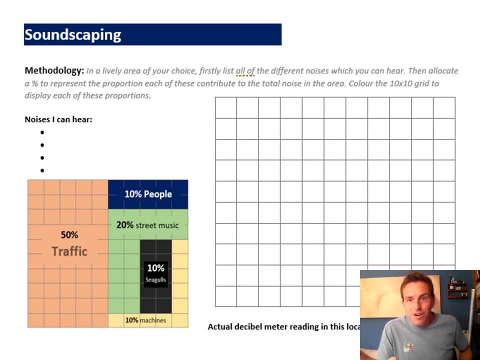 with the area around you and you just try and be as quiet as possible for a few minutes and you start making a note of all of the different noises that you hear and hear that are kind of contributing to the overall background noise that is present in that area. now, obviously, depending where you are- whether you're in an urban area or a more- 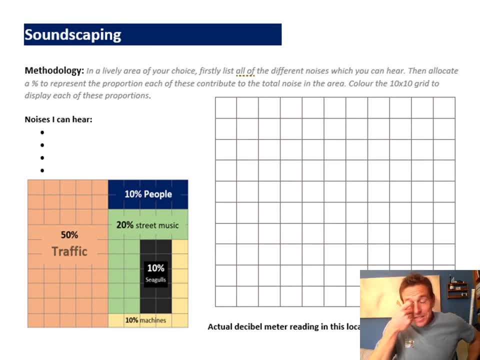 natural, perhaps countryside area, those noises are going to be different, and it might well be that in urban areas, you would expect those noises to be more man-made, more artificial. but your first challenge is to write down all of the different noises that you can hear. then, and this is where 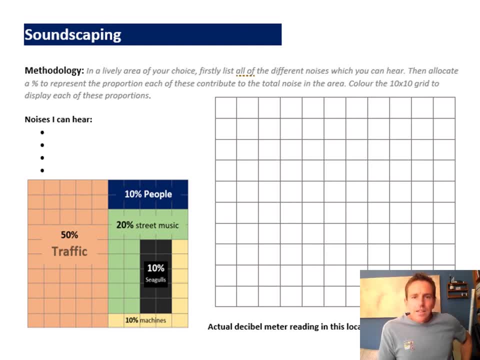 it is less scientific, approximately try to attribute a percentage to each of those noises in terms of how much out of the total noise that you can hear that they are contributing. so you can see in this little example that we've got here on the left hand side that 50 of the noise in this location. this person considered 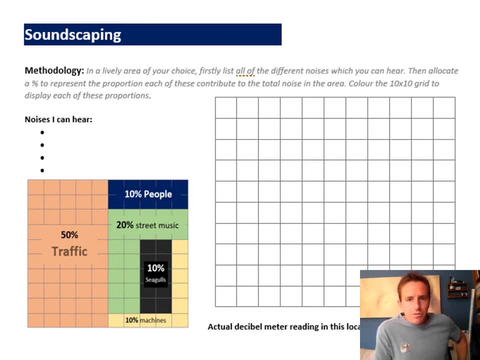 to be made made up from traffic 10, from people talking of street music, seagulls and also machines, obviously somewhere in the background too. so they've presented that on what's called a tree map, which is a little bit similar, i suppose, to a pie chart, it's just a different shape. 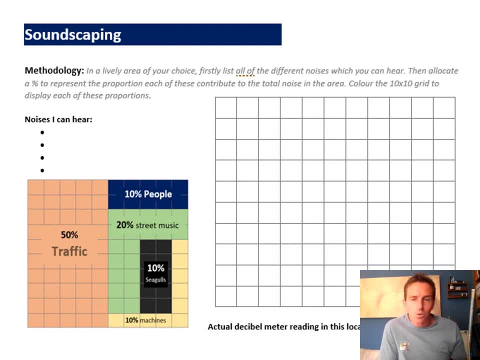 of the tree map. so you can see that the tree map has a lot of different sounds in it and the tree map in the middle has got a hundred squares in it representing the percentage that you're allocating to the contribution of each of these different sounds. that is a very nice visual way. 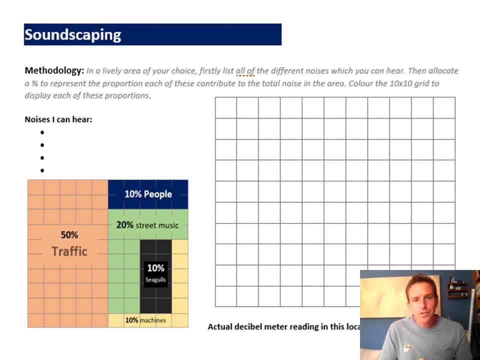 of presenting the noises in different areas. and again you could perhaps have a base map or an aerial picture, for instance, and then you could layer on these tree maps and draw a line to where you've done that survey to show how you've done that environmental survey. or maybe, if you're looking at the environmental impact of a 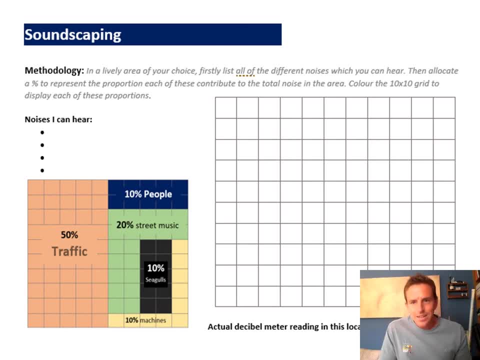 development, for instance. now this in its own again, is quite unscientific, unreliable- reliable in terms of its accuracy. so one of the things that you could do to enhance the accuracy of a soundscaping is use a decibel counter or decibel meter on your phone, and these are free to download. there's one. 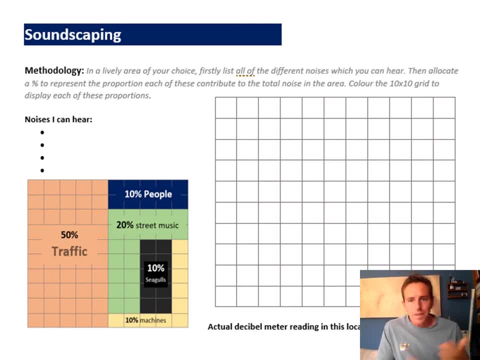 built into the jogger app as well, if you're going to use that. what they do is they use the microphone on your phone to gauge and to record the sound levels in the area that you're in. so if you're doing a soundscaping survey, you could also then once. 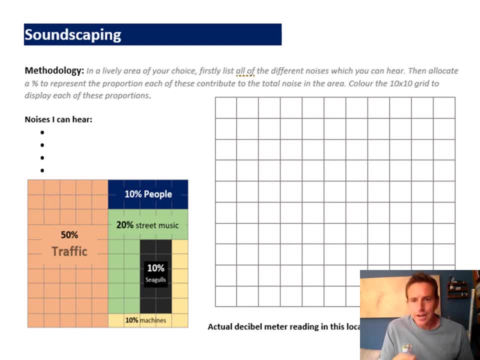 you've done that: gather the actual accurate decibel reading for the location that you're in. so to do a decibel reading, you'd need to set a time period: might be one minute, might be two minutes, might be longer, might be that you repeat it several times, but ultimately you'd come up with your final. 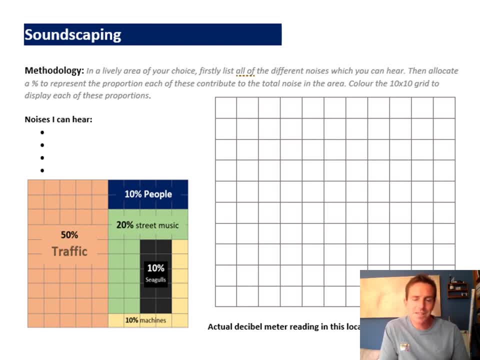 decibel reading that represents the sound levels in that location. you could allocate that to the tree map for that location as well, and then you could repeat that in several different locations. so again, it's trying to enhance the accuracy and reliability of the data that you're collecting. 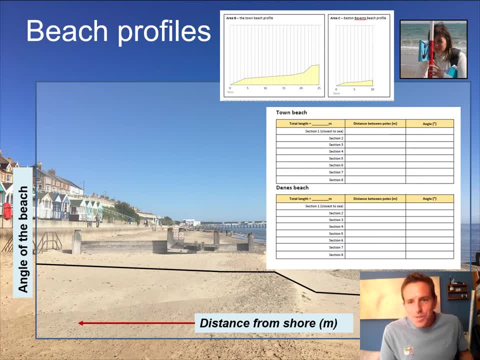 a beach profile. this is an absolute classic again for lots of teachers that are taking their students to coastal locations. i wonder if you can name the bits of equipment that you need. that's a quick geography field work question. i'm going to give you five seconds to do that. 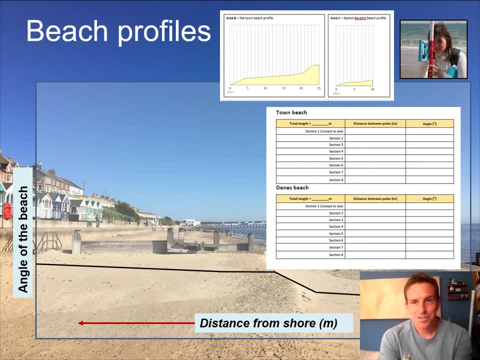 there's a clue up there in the screen: that student holding something there. all right, hopefully. you said ranging poles. those are the red and white- often red and white- sticks or poles that you you hold. you need two ranging poles to complete a beach profile generally. you need a tape measure. 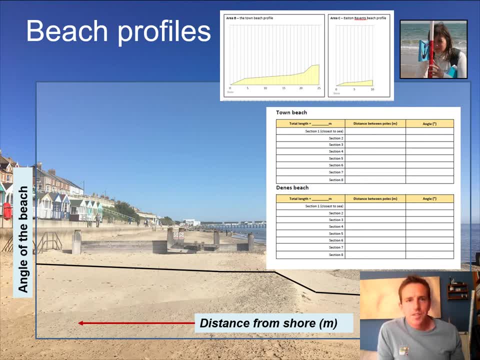 also, you need something called a clinometer as well, so i'm not going to speak in detail about how to conduct a beach profile. you'll be able to find that out from various different clips that already exist on youtube and also from the guide that the rgs have got, have issued. but the reason 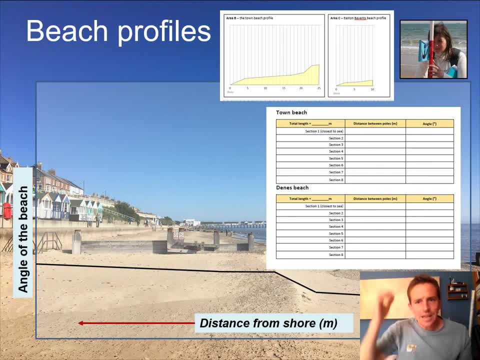 i wanted to show you this is that, for beach profiles and for a number of the methods of data collection that you are choosing, one of the things that i would suggest that you do is to take a photograph of the beach profile, and then you can take a photograph of the beach profile, and then you 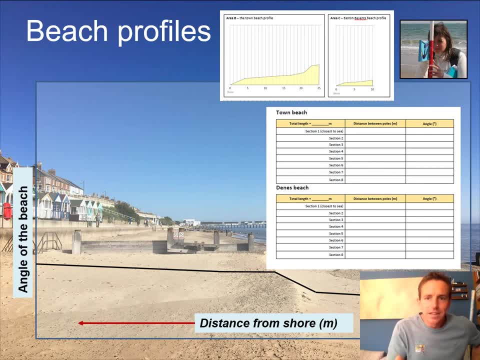 can take photos for the survey of the thing that you're investigating as well. so if you're doing a clone town survey, make sure that you've got a picture of that high street. if you're doing property quality survey, take pictures of the residential streets that you're investigating. 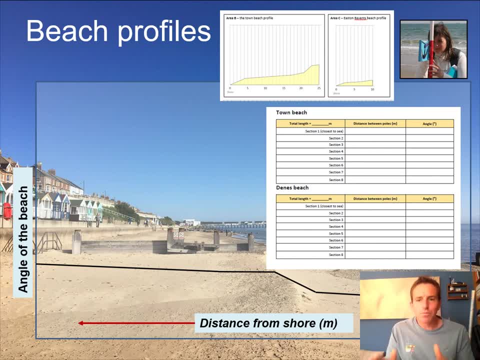 if you're doing a beach profile, which is where you're trying to draw a graph, essentially to represent the profile of the beach, why would you not also take a picture of the profile of the beach? and it might well be that you could layer the one on top of the other, or you could. 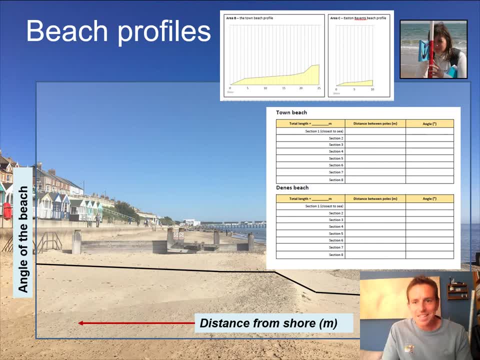 about the profile of the beach. so these things in your pockets, these mobile phones, are absolute assets, and don't be told that they're not. they can really contribute to geography fieldwork. they can enable you to take pictures, they can enable you to record sound levels, they can enable you to record interviews and 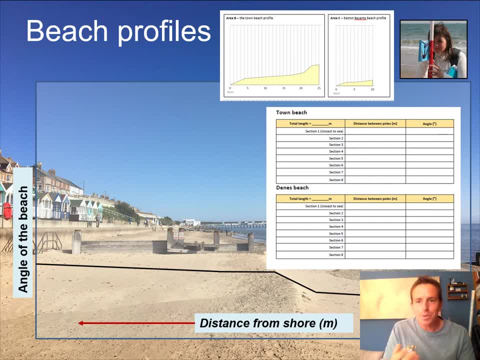 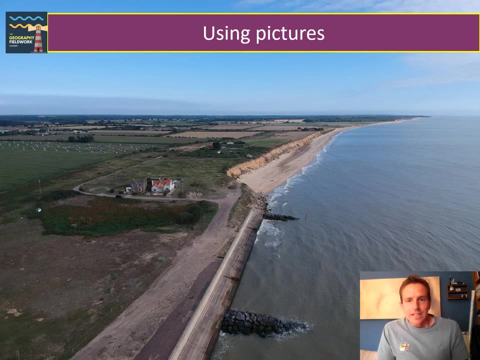 obviously, using the apps that we've developed, they can enable you to gather a huge amount of information as well and store that electronically. so don't be afraid to use the technology, as well as the classic technology that you are encouraged to use when you do work, and, with that in mind, it might well be some. 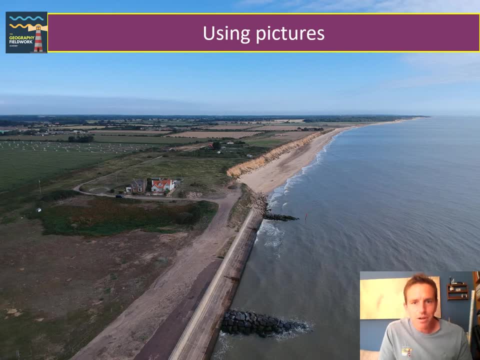 of you, if you're very lucky, might know somebody that's got access to a drone. who might know somebody that has taken pictures of a particular place aerially but has got a nice camera and it doesn't have to be up in the air, but it could be. 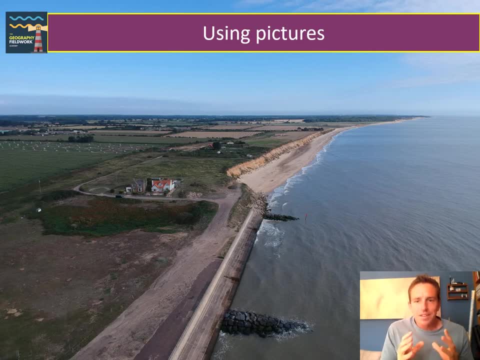 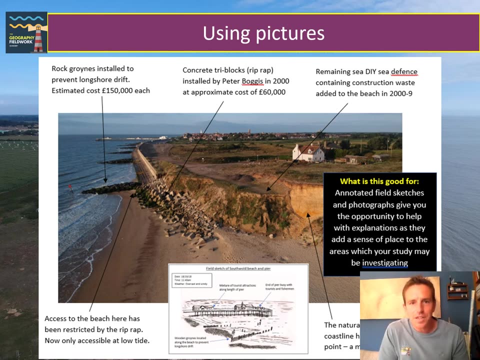 just ones that are mounted on the ground, but using pictures and using field sketches are a really useful thing to still do in a geography study, and they are things that enable you to annotate and bring the fieldwork location that you're investigating to life. so, no matter what your study is, I would suggest that you 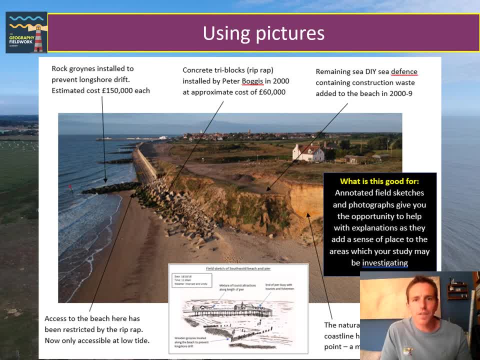 do include field sketches or photographs of the location that you're investigating, that you annotate these pictures and you really use them to bring the area to life, as I say. so it might be an idea, like we've got in this little field sketch down there in the middle of the picture, and then you can. 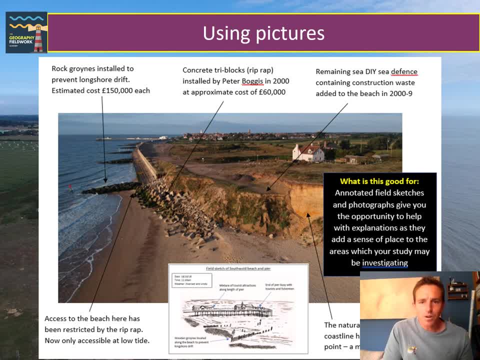 see that you've got a picture of a field sketch down there in the middle of the screen, but you make a note of the time and the date which you did your photograph or you did your field sketch- perhaps the weather conditions and any other kind of external factors which might be relevant, and that perhaps you 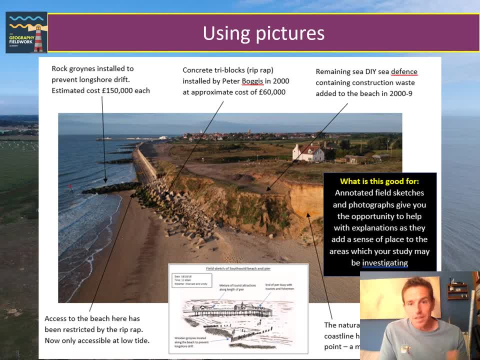 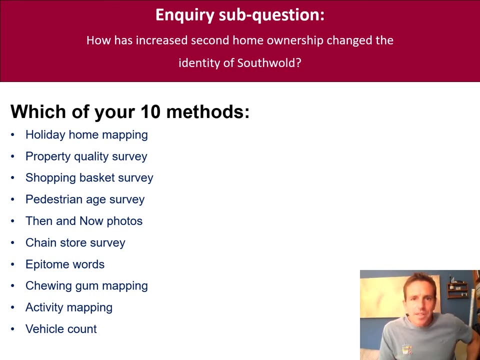 put a title as well to show exactly where that location is. it might be that you take the latitude and longitude coordinates of where you've taken that picture or that, done that that drawing from as well. so there you go. there's a few ideas. do as part of one of the A level courses in Southwold with students who are trying to kind of 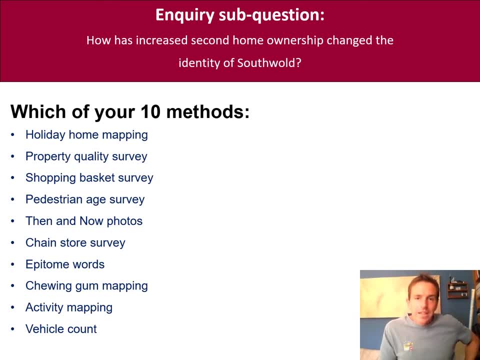 increase their understanding of field work is we do an activity where we give them an inquiry question, we give them a kind of an example sub questions. there's one there at the top of the screen: how has increased second home ownership changed the identity of Southwold? then we just 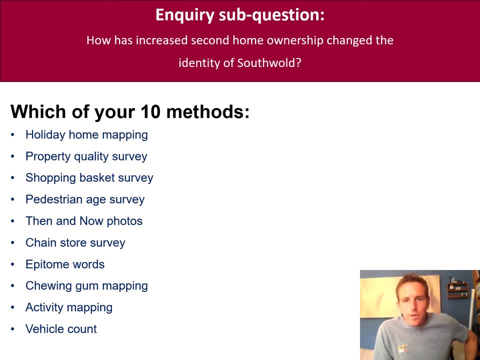 tell them to go off around the town and complete a range of different, almost random, methods of data collection. this helps them obviously learn more methods of data collection, but one of the things that we then ask them to do once they come back into the classroom is to then try and be a bit. 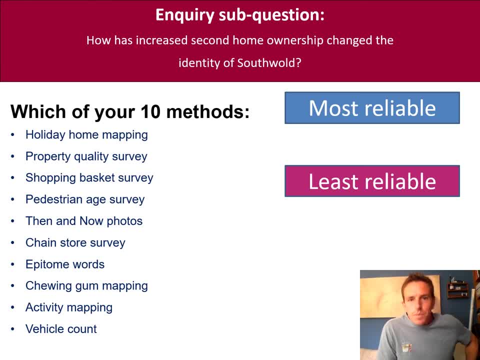 reflective and to think about how reliable those bits of data collection are. so this is one of the things that, when you're doing your planning, you're going to need to try and think about: is the data that I'm collecting reliable and, if not, how can I make it more reliable and more useful? 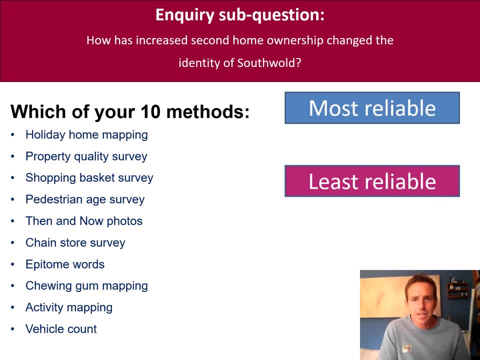 how can I make it more accurate? what are the things that are affecting its accuracy? how can I make it more reliable and more useful? I make it more accurate. and the other thing which is probably at this stage more relevant, particularly at the early planning stage, is which bits of data collection that you're planning to do are actually relevant to the question that. 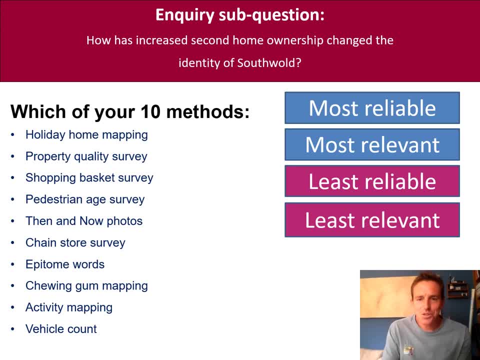 you've been given. so one of the things you've got to ensure is that when you're doing and taking the time to plan and to conduct field work, that the results and the the field work that you're completing is actually helping you and is going to be answering your study, because if you're 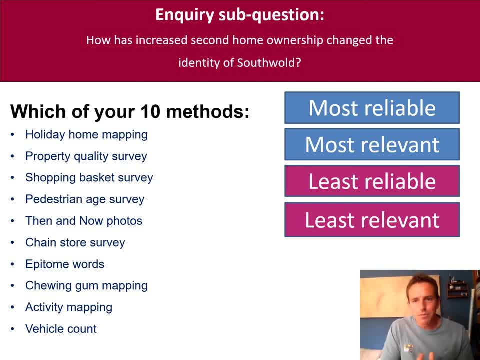 doing something and it actually isn't relevant to the study. really no point in doing it at all and spending any time on it. so we've, we tell these students to go off and complete their 10 surveys, and then we kind of redirect them back to the sub-question that we have set them, and then we 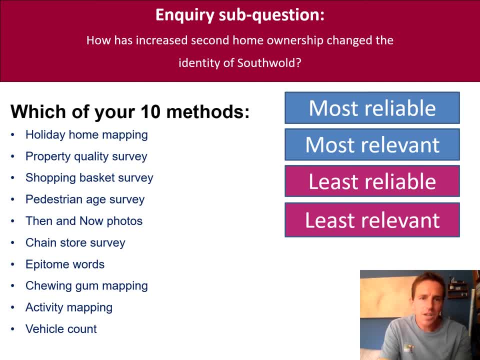 give them the challenge of them being reflective and thinking about, then, which of these methods that you've just done are actually relevant and helping you answer that sub-question, and that then encourages them to critically reflect on the what they've done and actually think: well, actually there's no point doing those. there's no point. 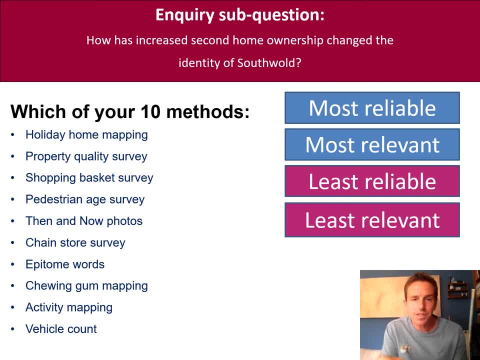 doing that one or that one, but that one was really good, that was really relevant, and so too was that one. might well be that they just get it down to two or three of those methods and they pick those, and that, in a way, is kind of the process that you've got at the moment. you hopefully now will. 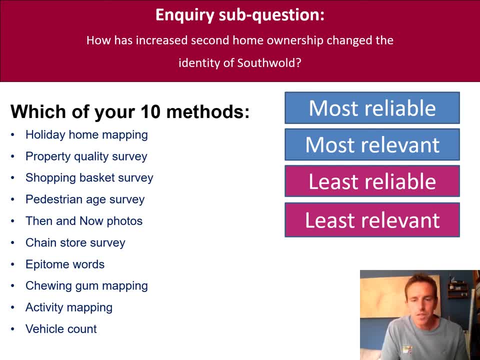 go out and look at the different methods of data collection that are available to you, the things that you can pick off that menu, almost of field work. you then look again at what your sub questions are and you think, yeah, okay, that method would help me answer that sub question and that method. 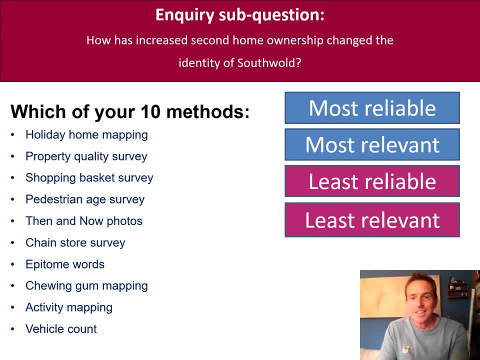 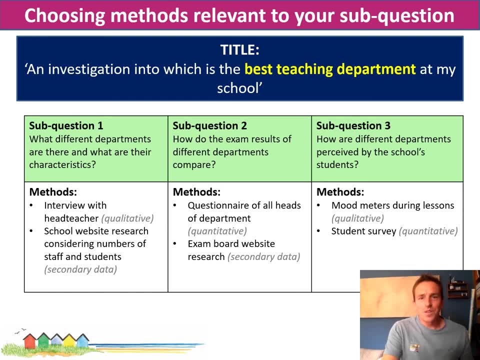 would help me answer that sub question. and that's the process now that you've got as your next challenge, so we're going to leave it. go back to this again. this is your holy grail. you've got, hopefully, here your title. you've got your supporting sub questions. this is the bit now that 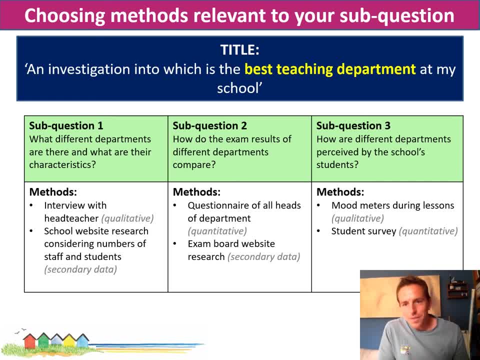 we're encouraging you to do is to think about what methods of data collection that are available could you do to be relevant to those sub questions and if there aren't any methods you can see that are available that you're kind of already being talked about or on jog it, or on the rgs guide or on the documents. 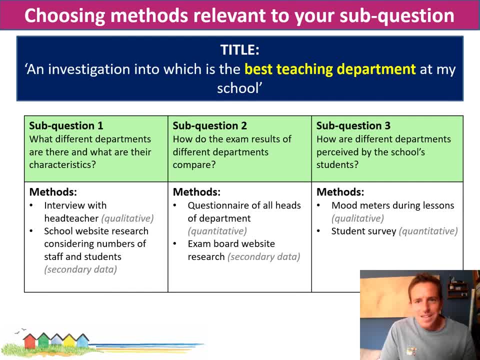 that you can access from anywhere else? are there any methods of data collection that you can create that can be completely bespoke to you and, if so, come out of them, be creative and allocate them to the sub question that they are relevant to. so that's your next challenge. good luck with that, and we'll see you for the next one.